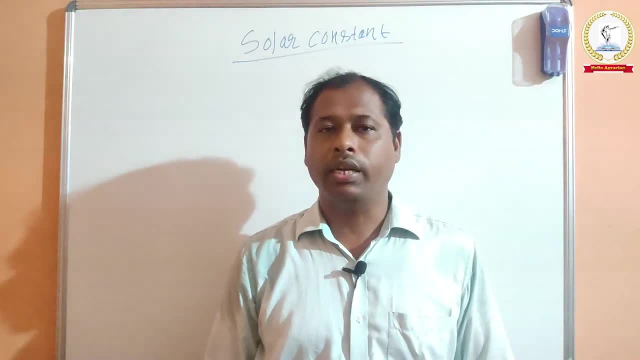 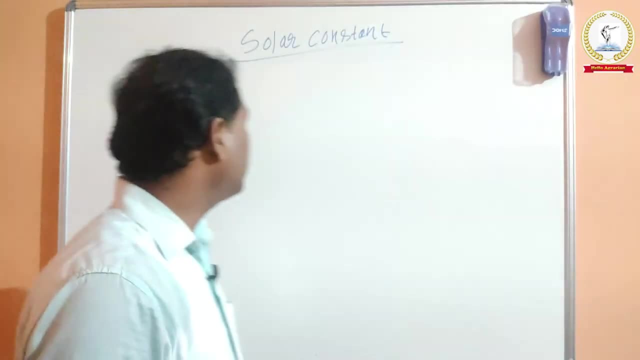 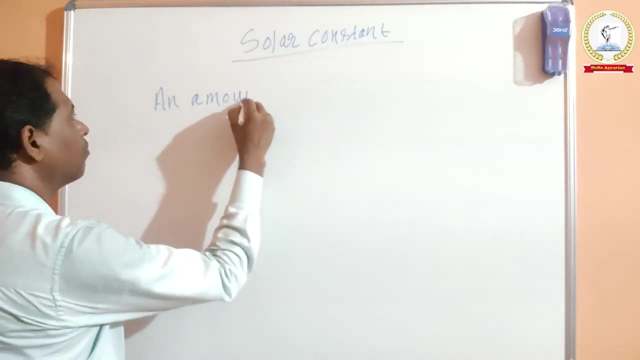 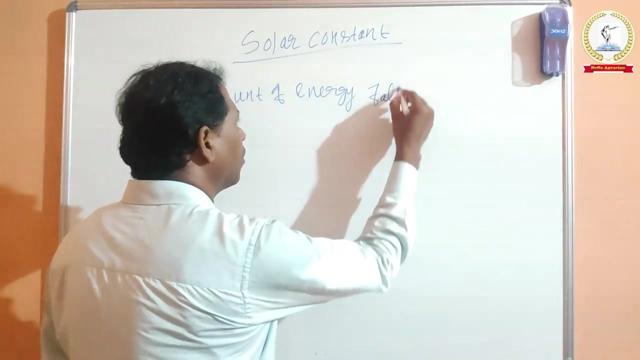 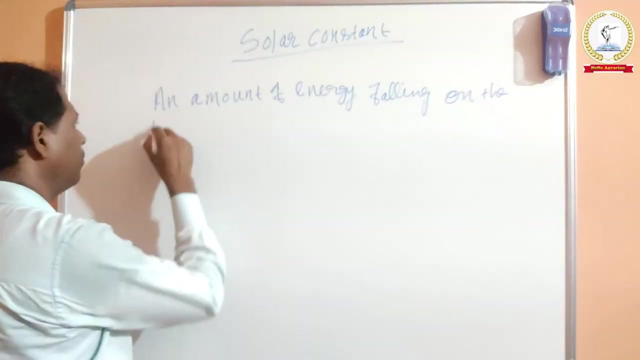 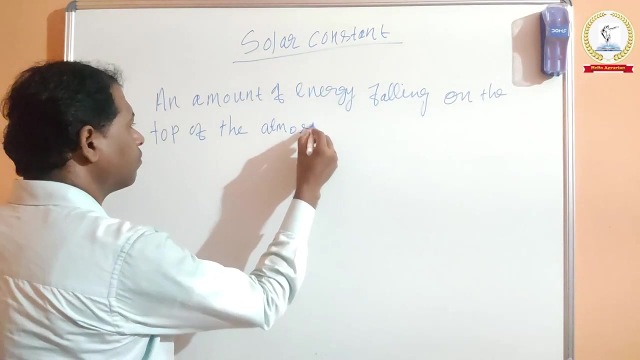 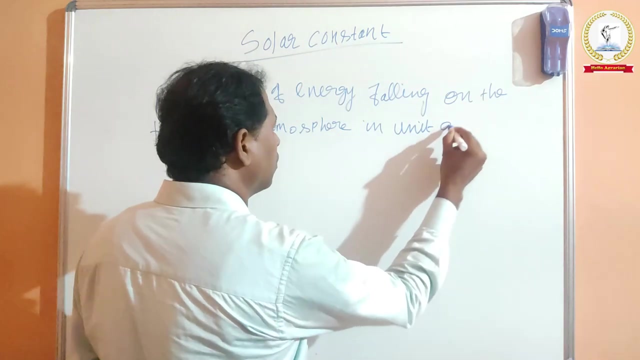 We can define solar constant as amount of energy falling on the earth's surface per unit area, per unit time. So we can define solar constant as. solar constant as an amount of energy falling on the top of the atmosphere, in the atmosphere. So we can define solar constant as. 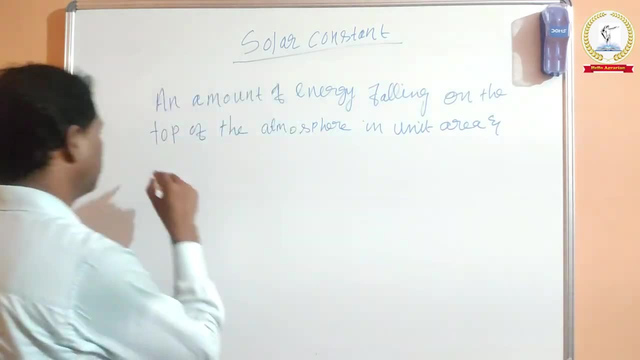 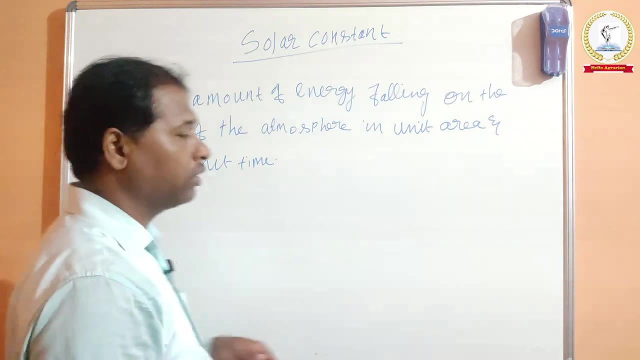 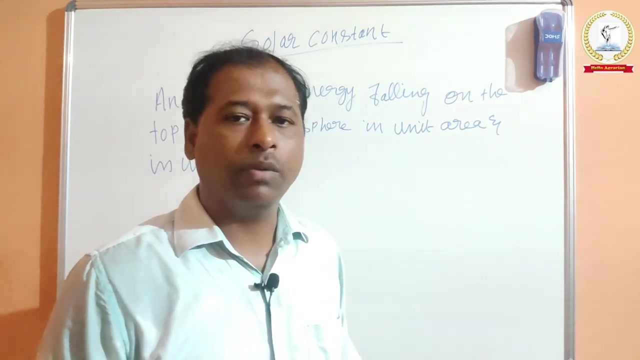 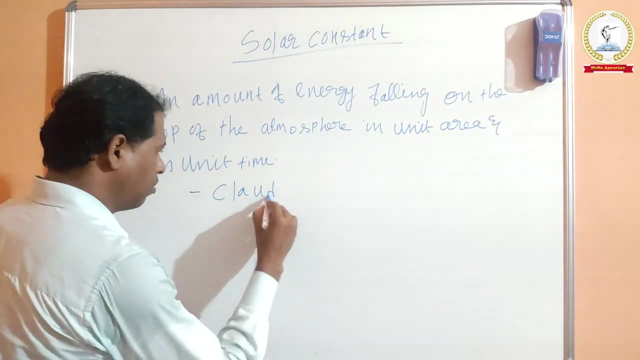 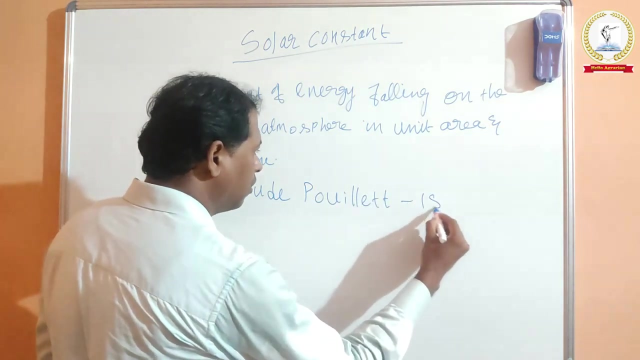 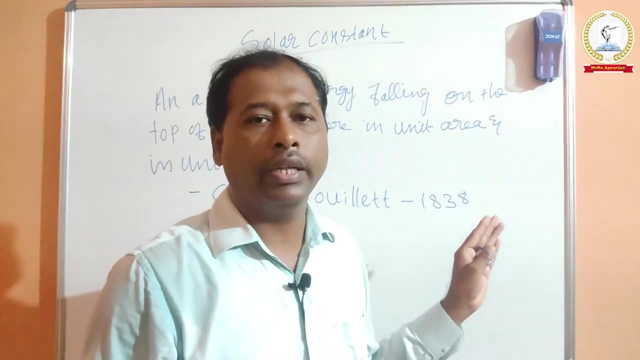 unit area and in unit time. So it is called solar constant. This solar constant first time estimated by Claude Paulet in 1838.. Claude Paulet, estimated by Claude Paulet in 1838.. Paulette in 1838.. He was the first person estimated solar constant in 1838.. 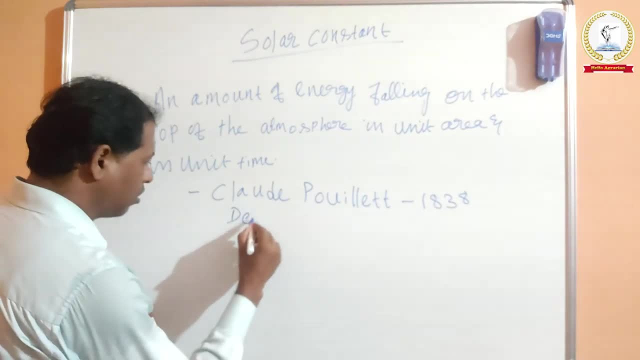 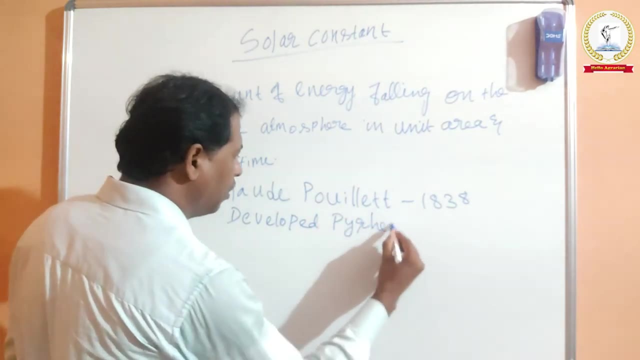 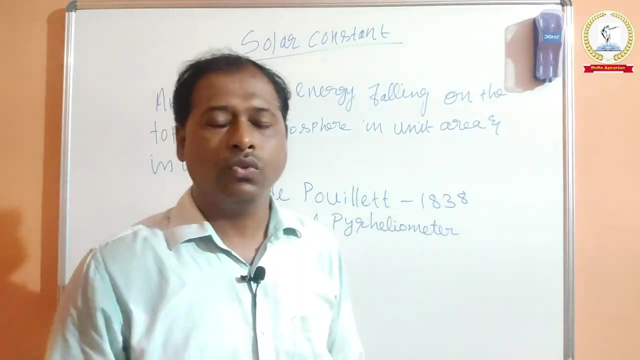 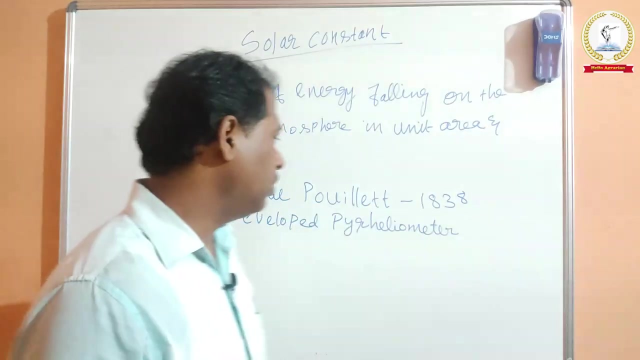 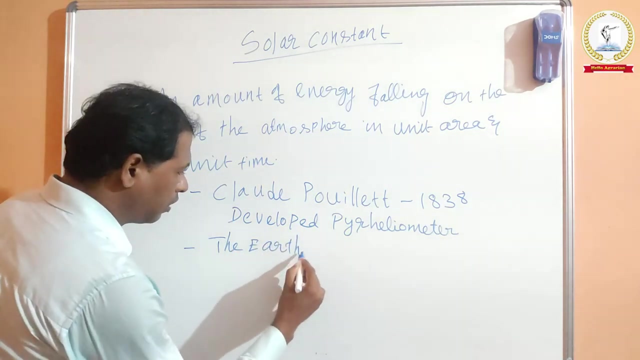 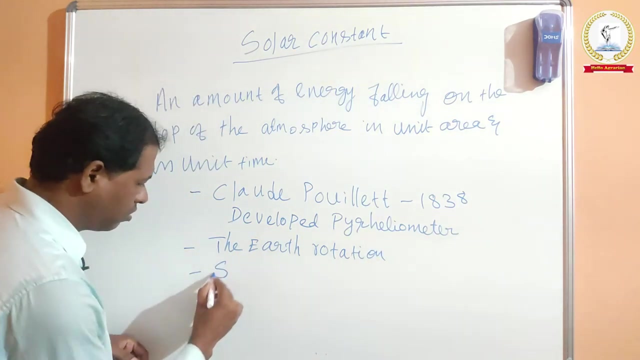 He also developed per-heliometer. He also developed per-heliometer in 1838.. You see, the value of this solar constant varies year round because two factors: one is the earth, the earth rotation, and the second one is sunspot cycle. 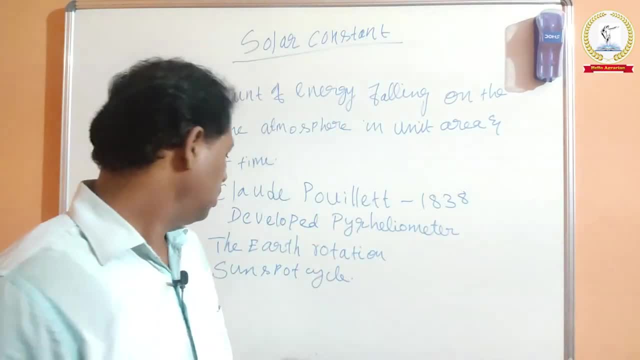 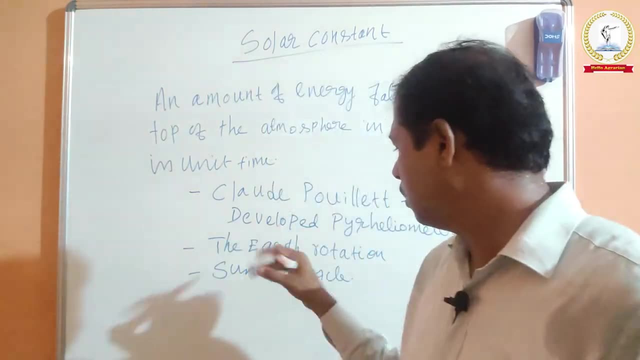 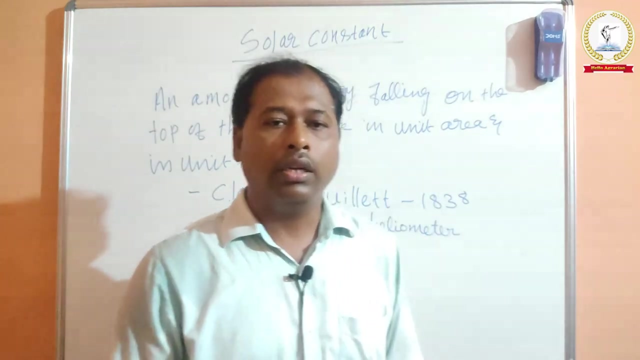 The first factor is the earth rotation. The second one is the sunspot cycle You look at here. in our last video also, we discussed this earth rotation. As we all know, our earth rotates on its own axis and revolves in an elliptical orbit around. 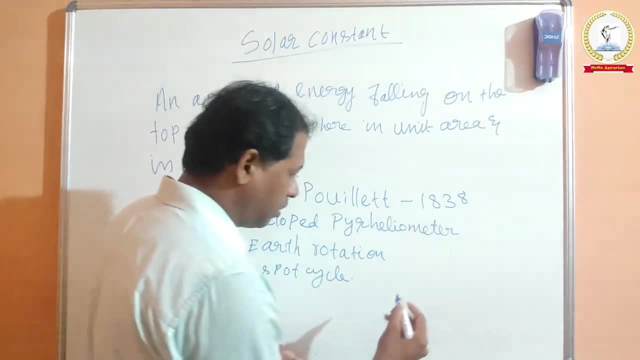 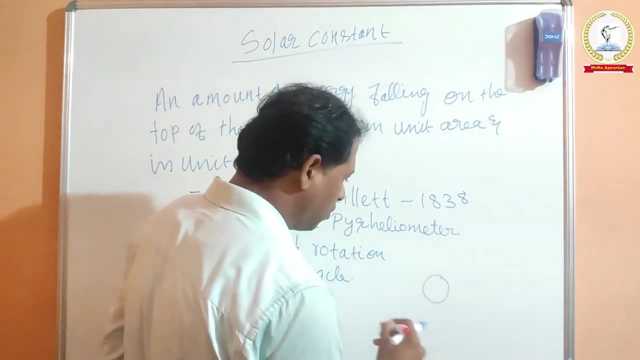 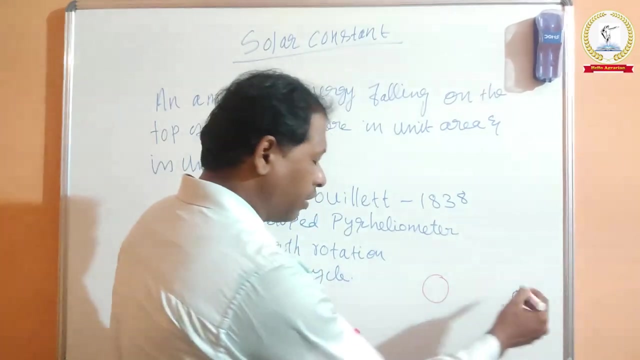 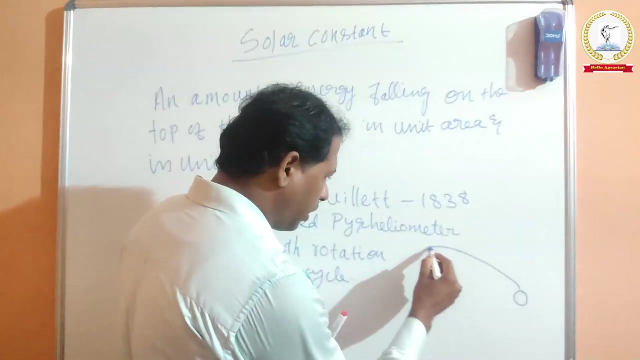 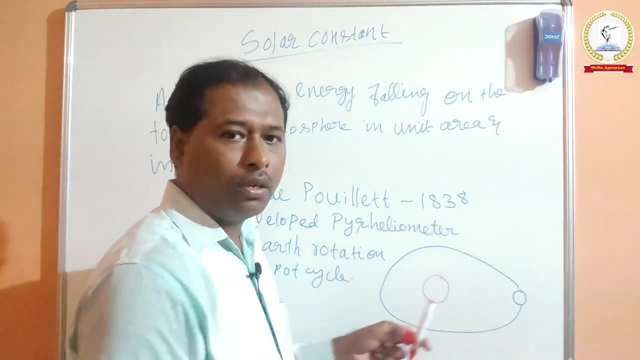 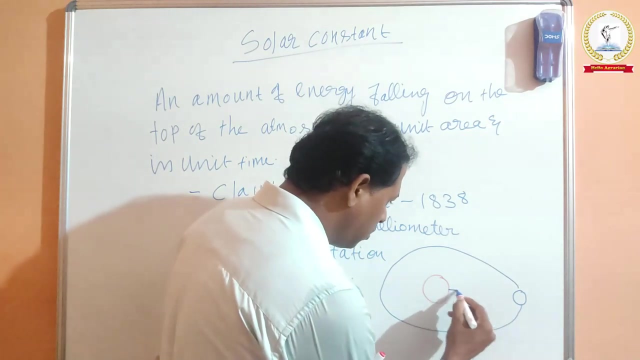 the sun. So suppose, for example: So this is the sun And this is the earth. So our earth rotates on its own axis and it revolves in an elliptical orbit. So when the earth comes closer to the sun, that is called perihelion. 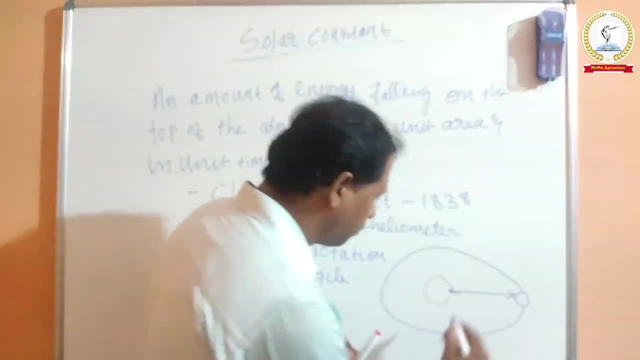 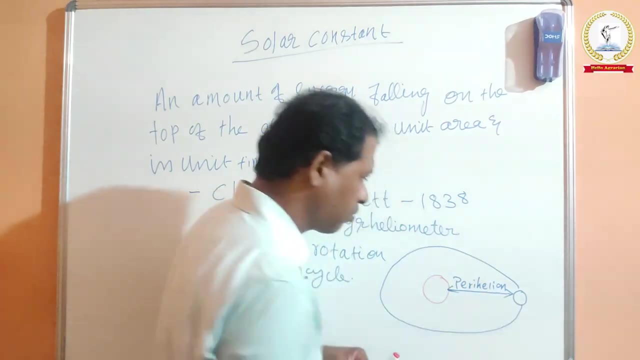 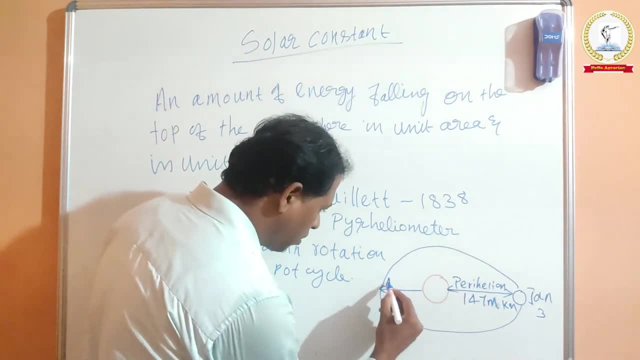 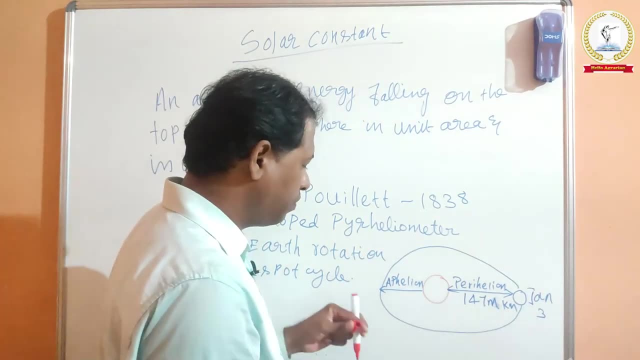 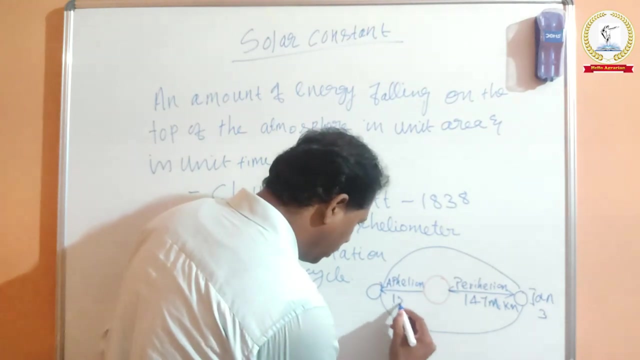 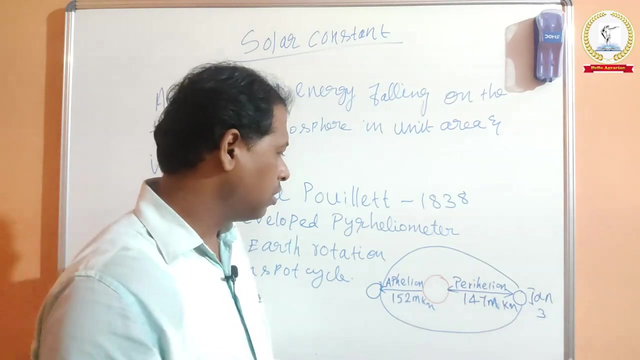 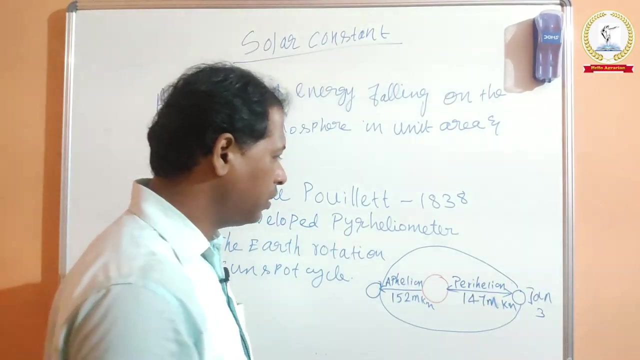 that is called epihelion. So during this time the distance between sun and earth is about 152 million kilometer. So because of this the solar constant value will vary. You see here. so our earth is in an elliptical orbit around the sun. In sun. it is in elliptical orbit around the sun. Certain part of the time our earth come closer to the sun, that is called perihelion, and sometime the earth goes away from the sun, So that is called epihelion. 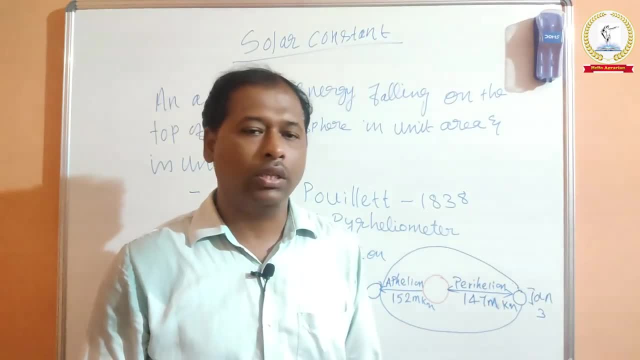 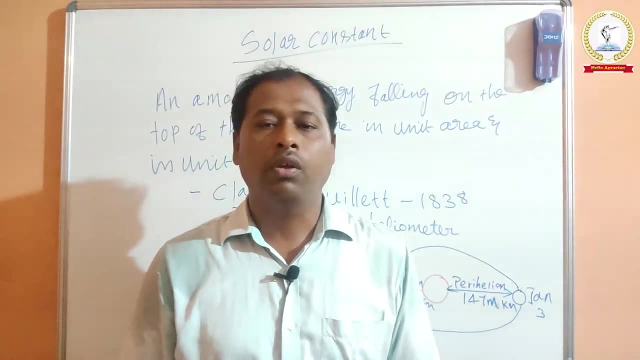 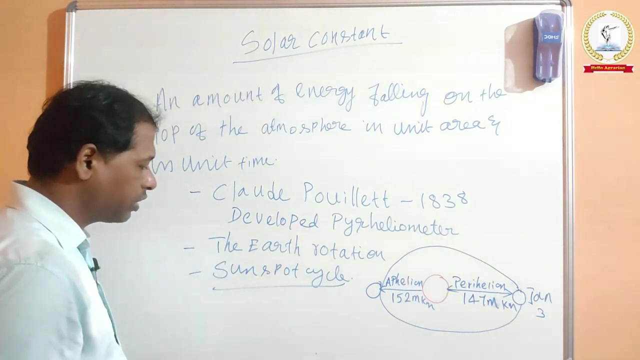 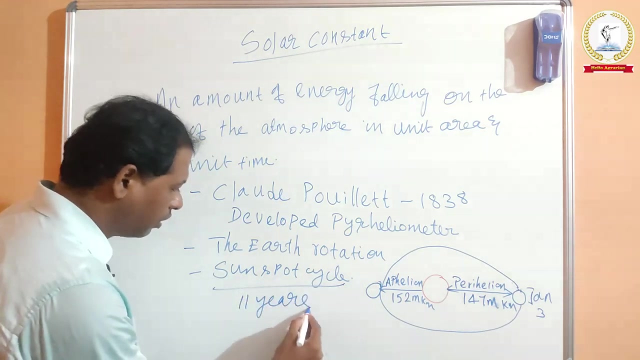 So, because of this, solar constant value will vary. Another factor is the sunspot cycle. Okay, so the sun output varies by 0.1 to 0.2 percentage During its 11 years of sunspot cycle. Normally, this sunspot cycle occurs once in 11 years. 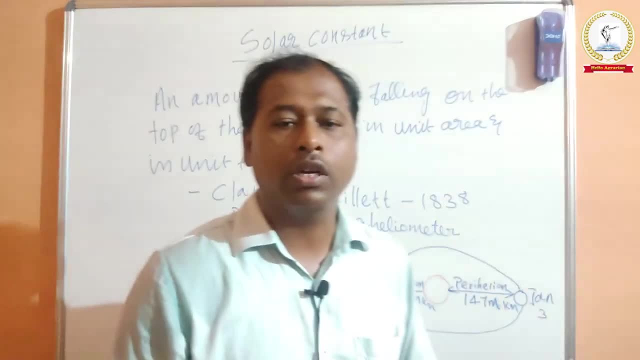 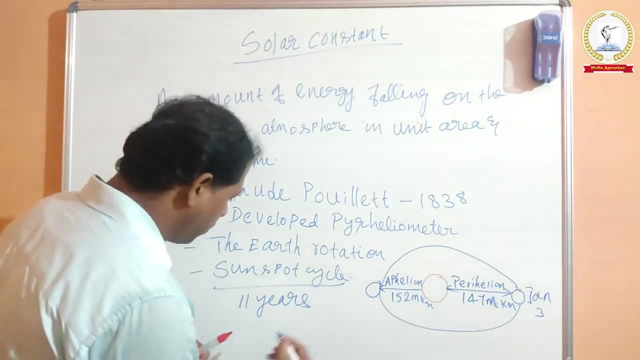 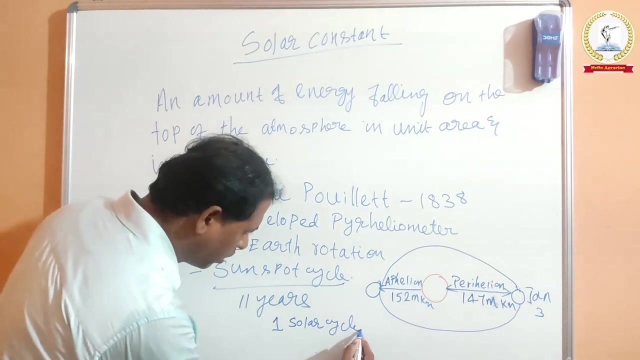 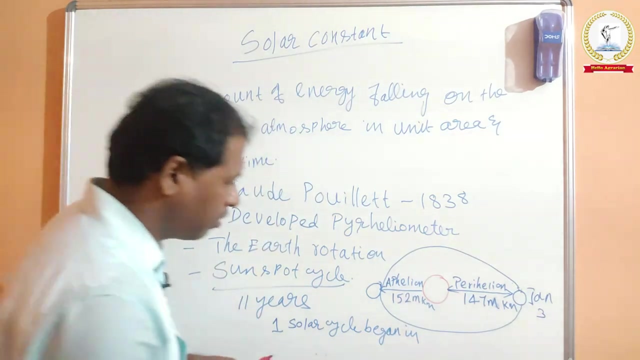 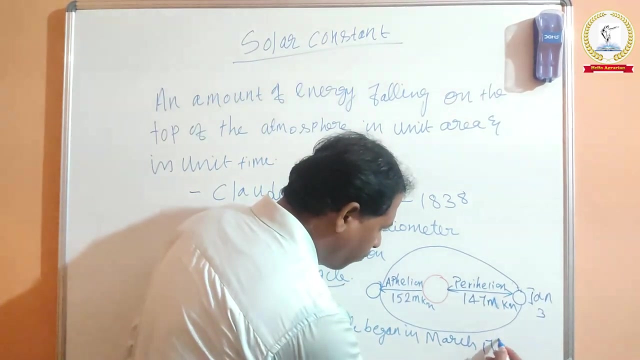 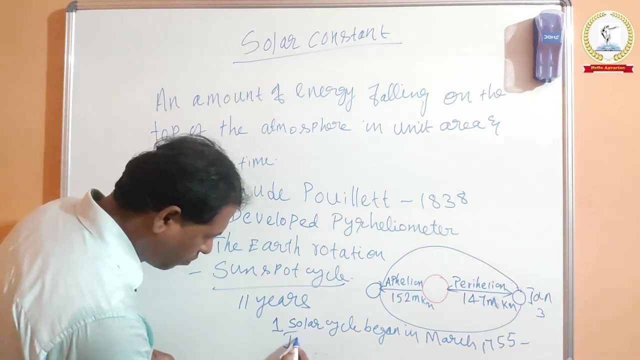 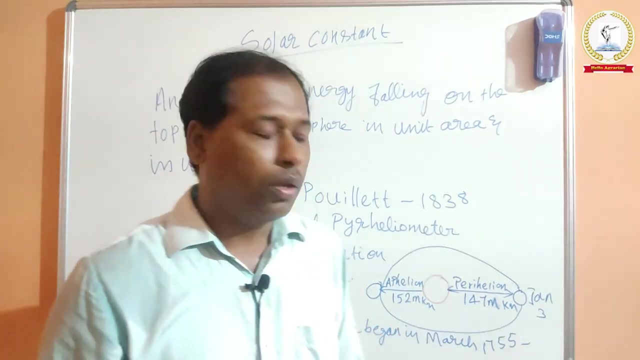 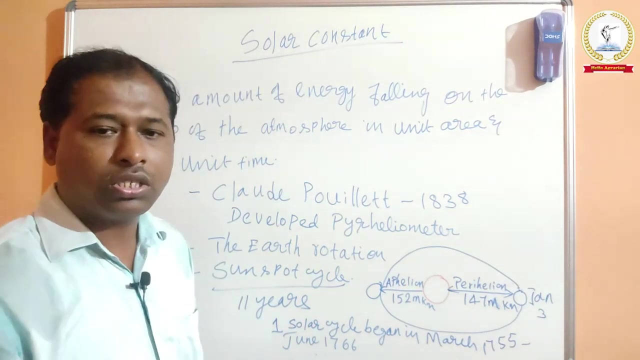 Okay, once in 11 years the sunspot cycle vary. The first solar cycle observed in March 1735.. The first solar cycle began in March 1755 and ended in June 1766.. So the first solar cycle began in March 1755 and ended in June 1766. 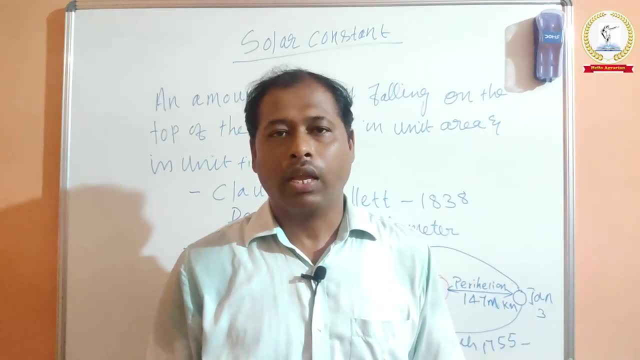 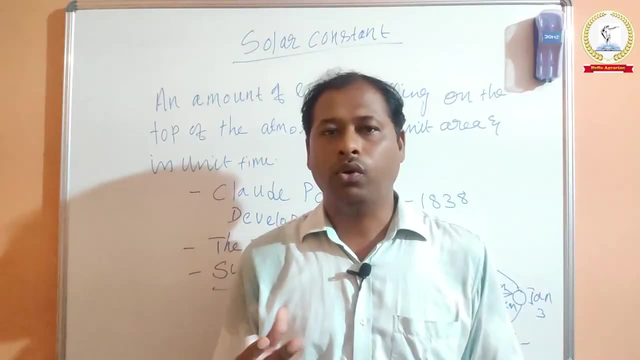 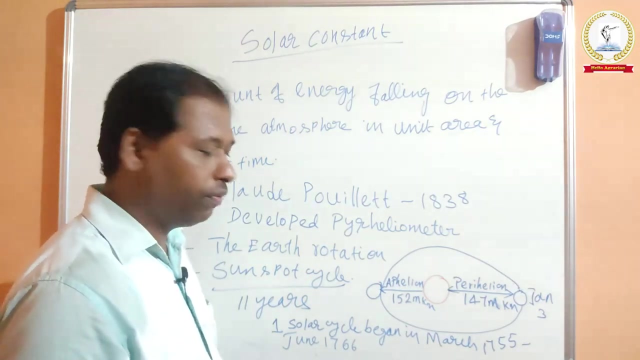 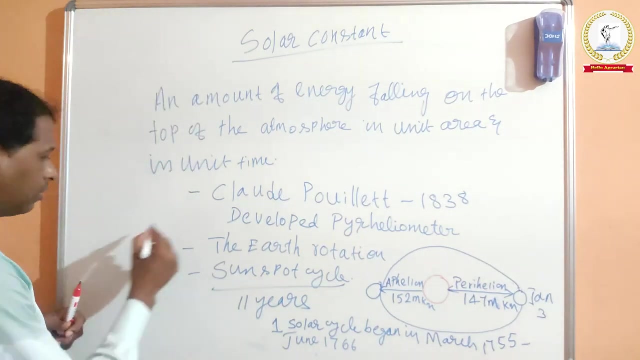 You see, our sun is a huge ball of electrically charged gas. So this charged gas moves. it produced more powerful magnetic field. So the first solar cycle began in March 1755. And ended in June 1766. And currently so at this time we are in. current solar cycle is 25th. 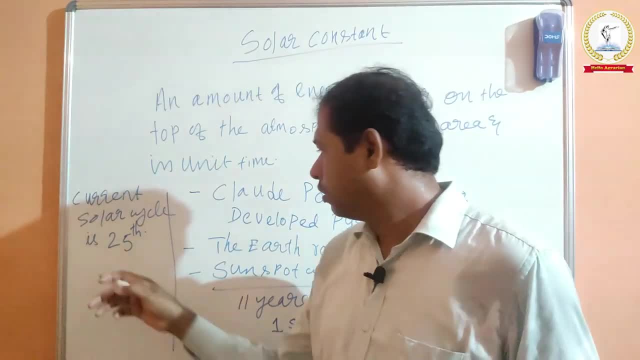 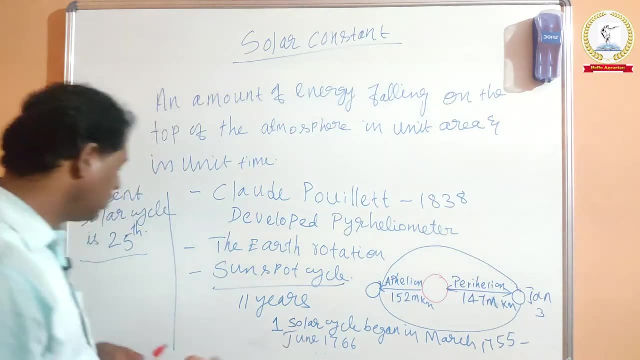 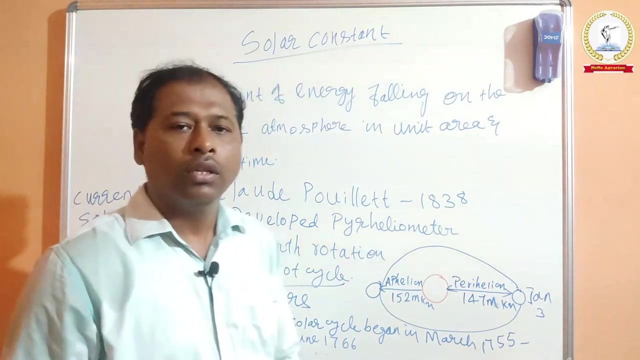 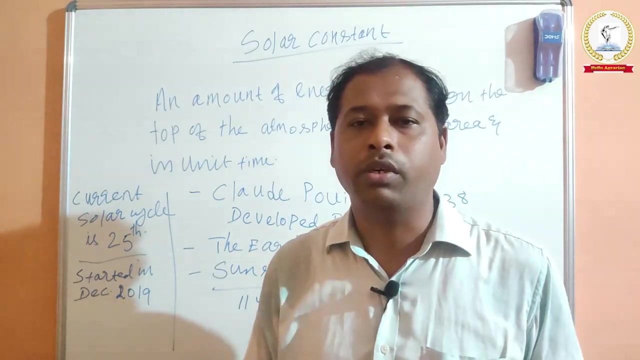 So we are in now in 25th solar cycle. The current solar cycle is 25th solar cycle. It was began in started in December 2019.. So at present time, we are in 25th solar cycle and it was started in December 2019 and it 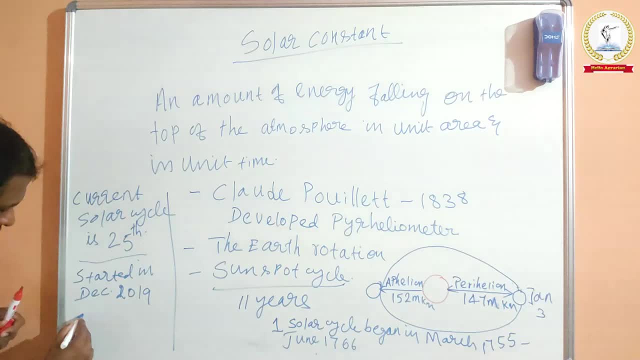 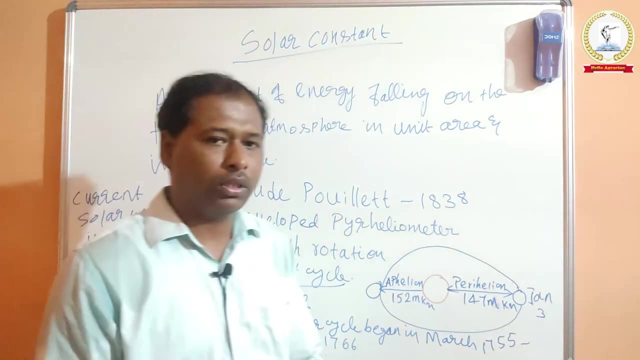 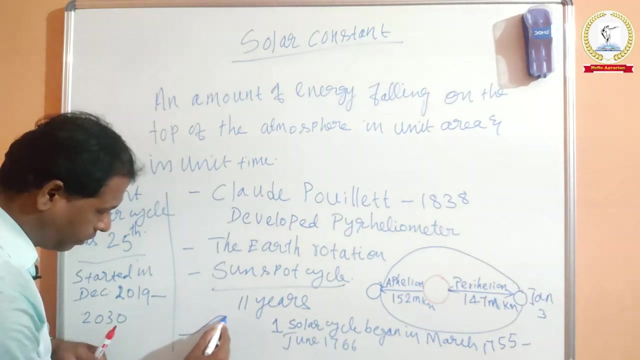 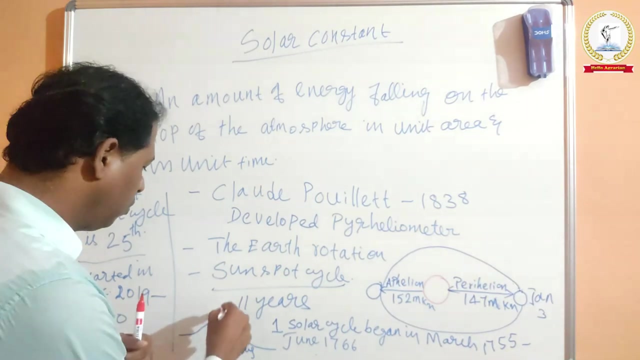 is estimated to end in June. So it is estimated to end in June. So it is estimated to end in June. During the solar cycle the sun emits lesser radiation. then it increase the peak, thereafter it decrease the emission. So around 5.5 years of the solar cycle it goes to peak, then it declare the emission. 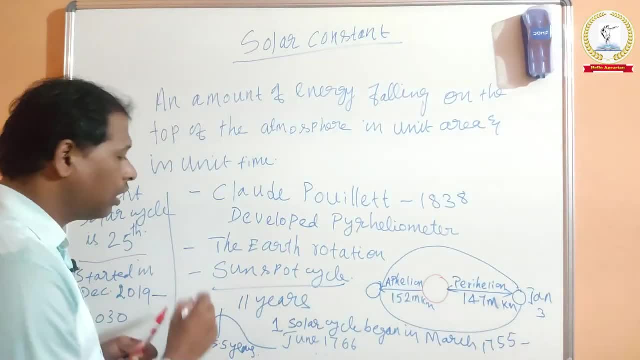 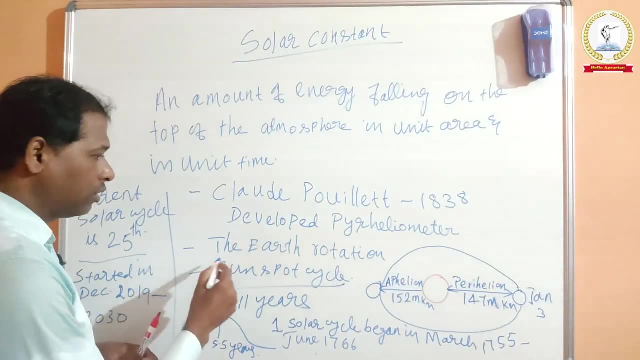 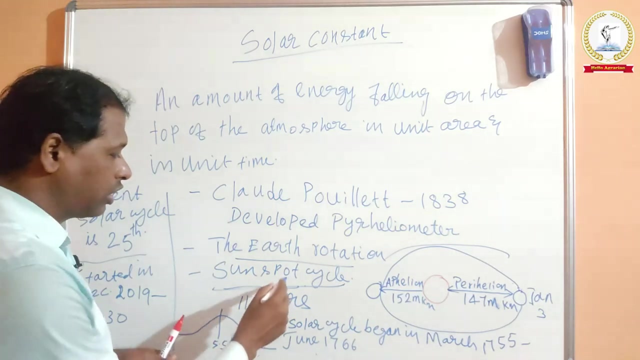 power. So this is because of this also the solar constant value vary. So there are two factors. one is the earth rotation- that what we discussed over here- and second one is sunspot cycle. So the sunspot cycle occurs once in 11 years. 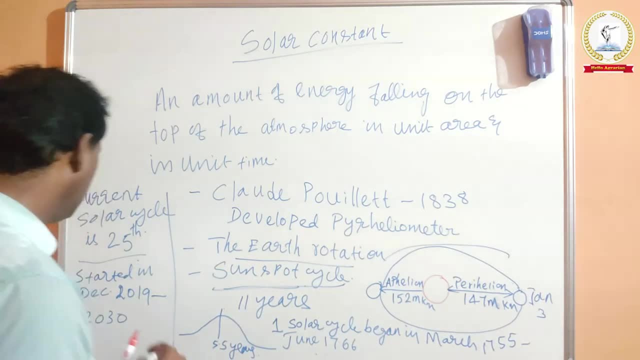 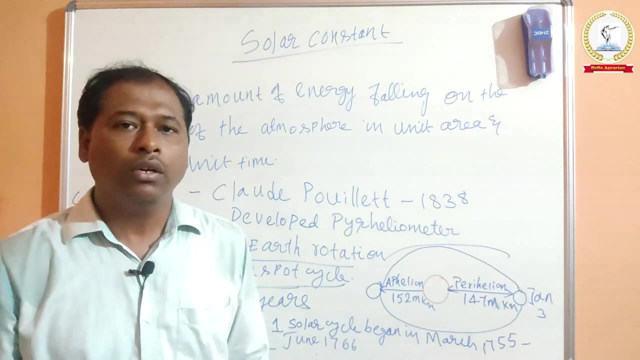 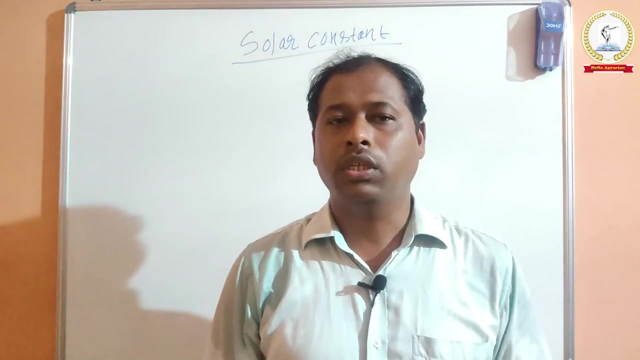 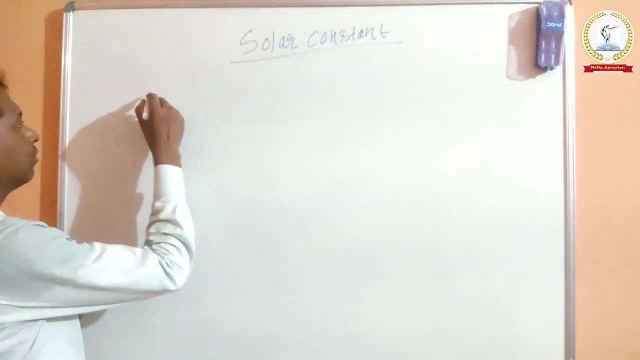 So now, currently we are in 25th solar cycle. it was started in December 2019 and it is estimate it is estimated to end in 2030. So I can delete this one. Next one is how to calculate the this solar constant. 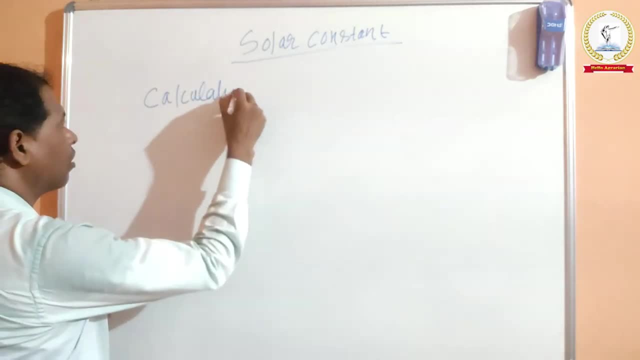 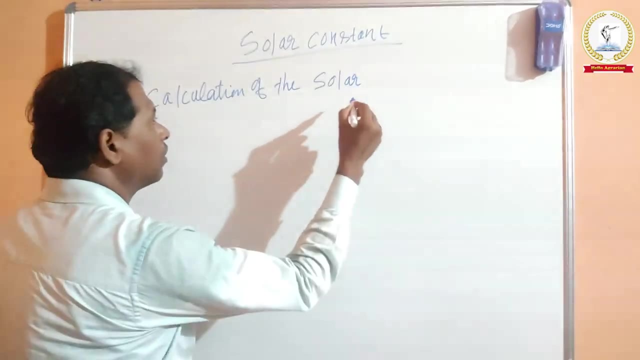 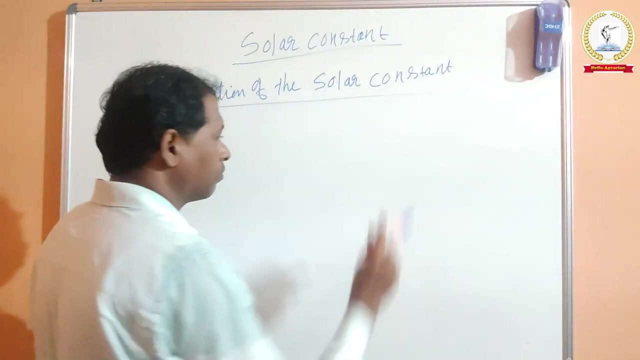 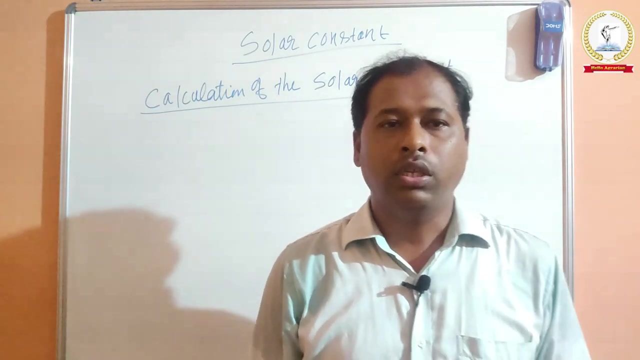 So calculations of the solar constant. So for calculating this solar constant we need two primary information. One is the radiation is incident and a perpendicular to the earth civilization, And this radiation isptic. Another one is the thought earth radiation is conjunct, The otheranco is non irritant. 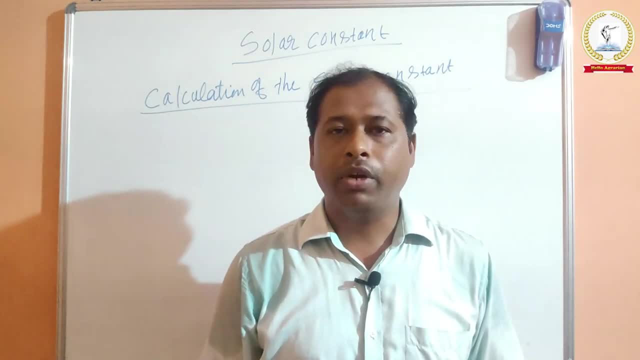 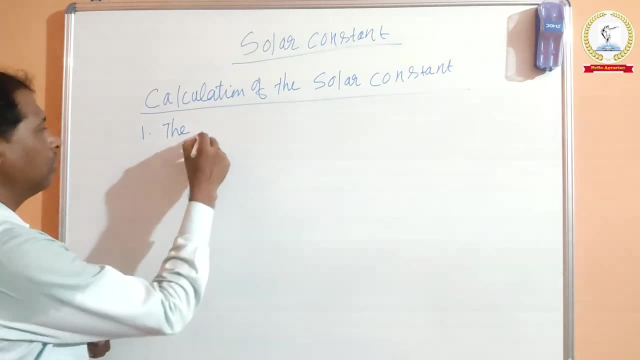 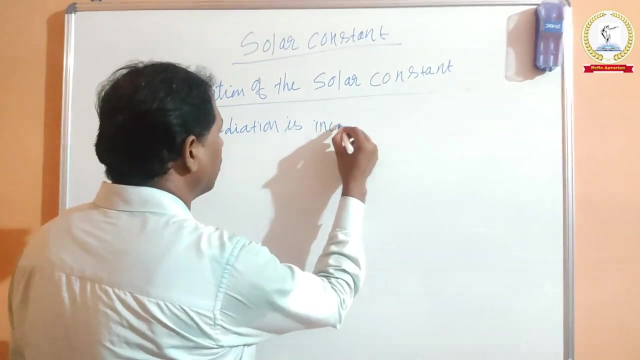 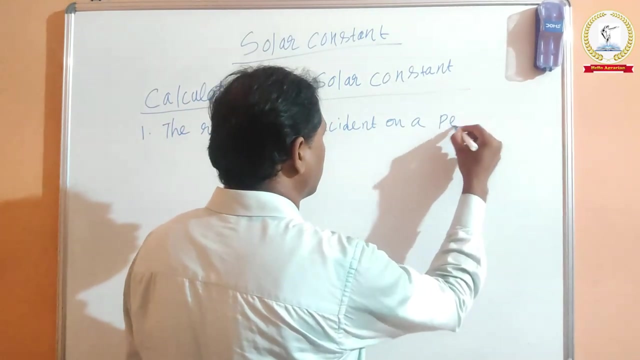 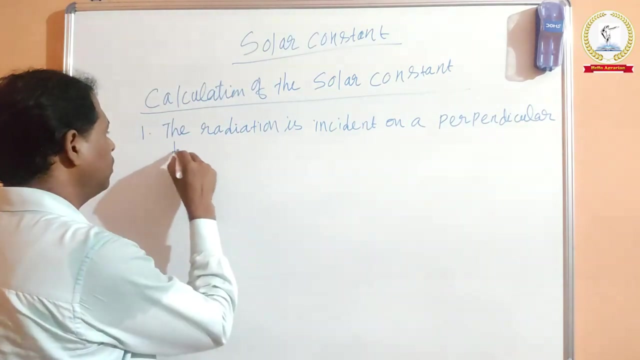 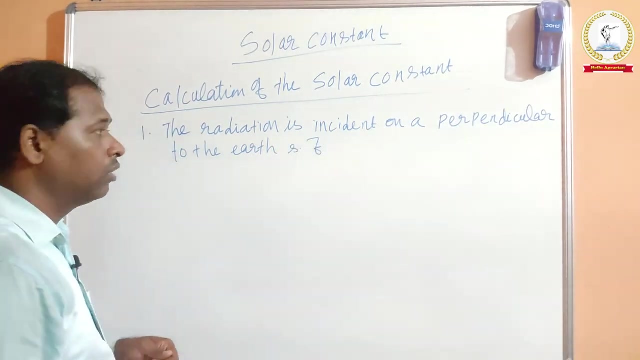 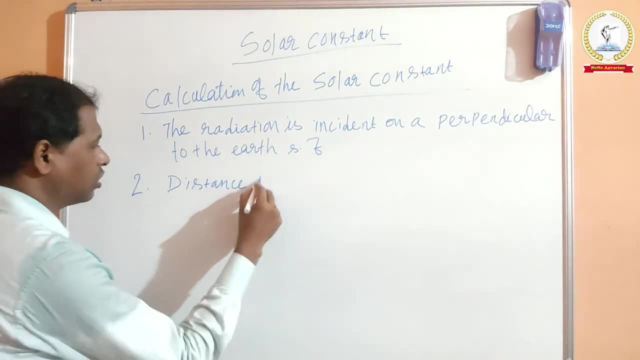 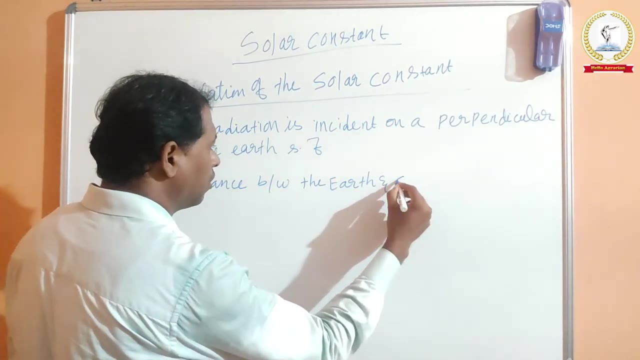 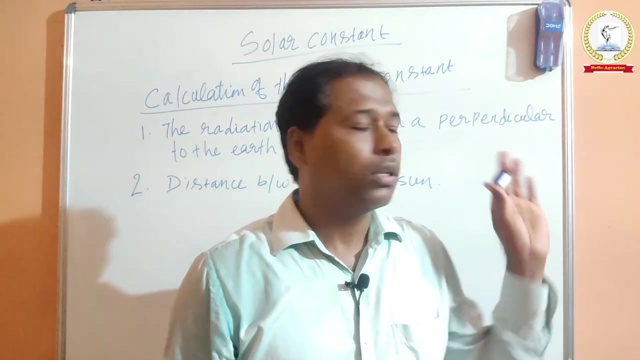 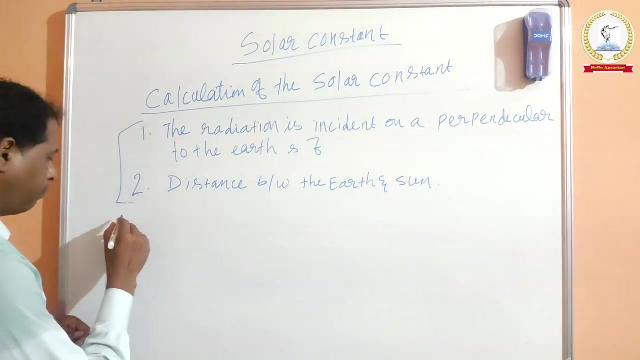 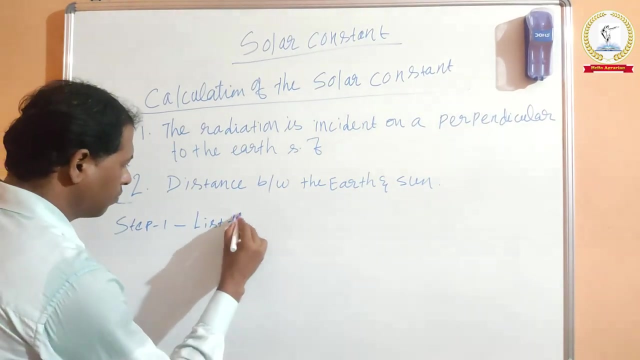 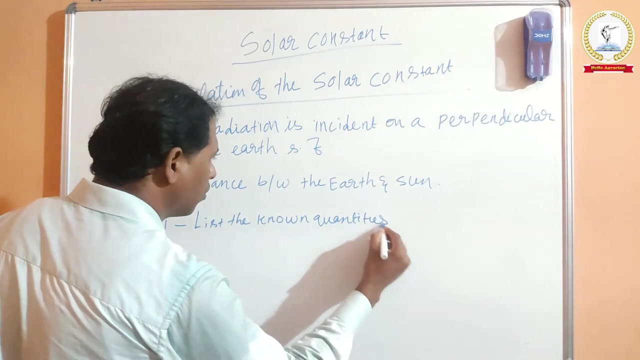 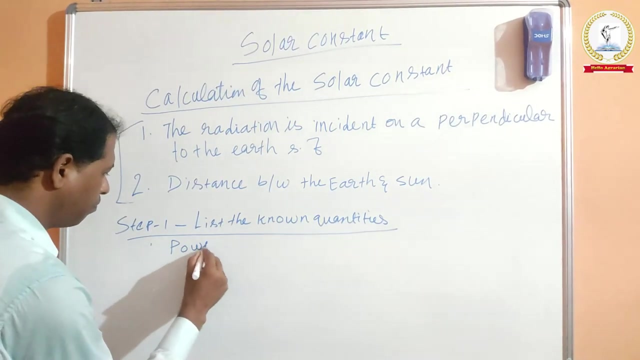 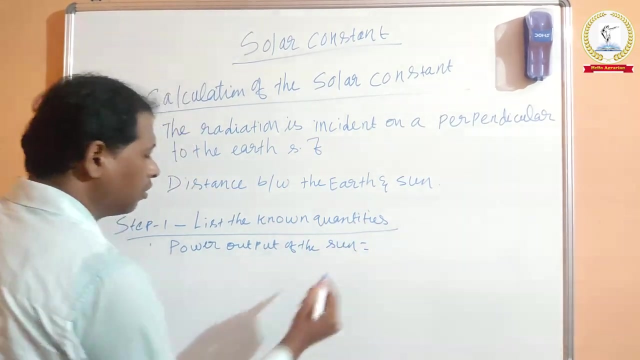 distance between the earth and sun. So these two information required to calculate the solar constant. There are four steps involved to calculate this solar constant. The step one is list the known quantities in this power output of the sun. So that is equal to: 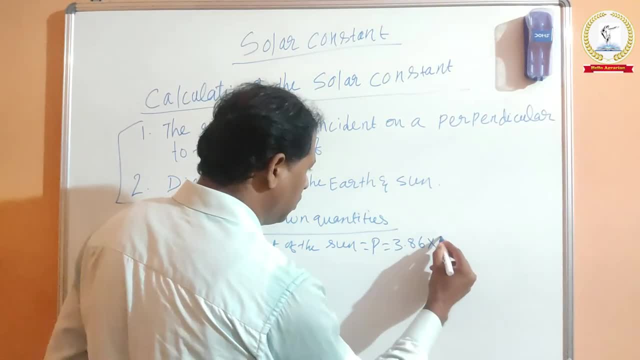 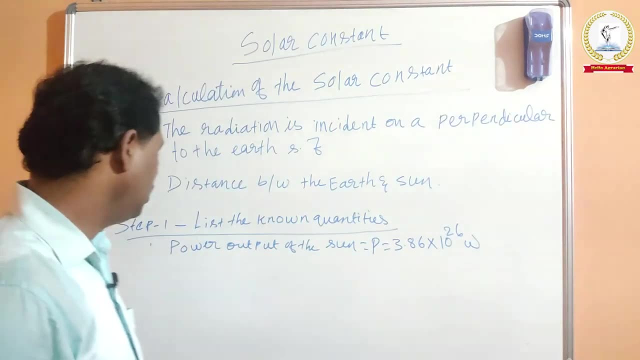 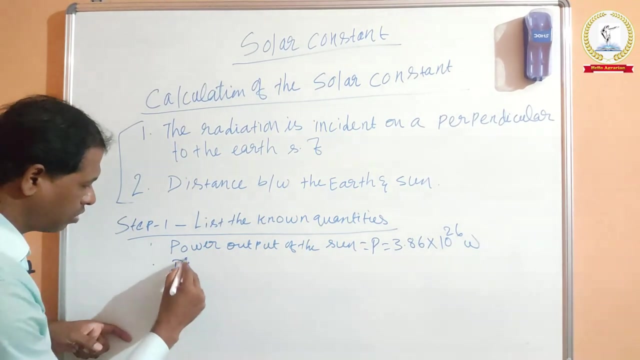 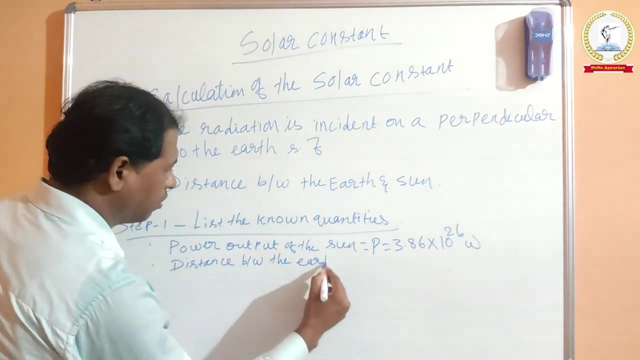 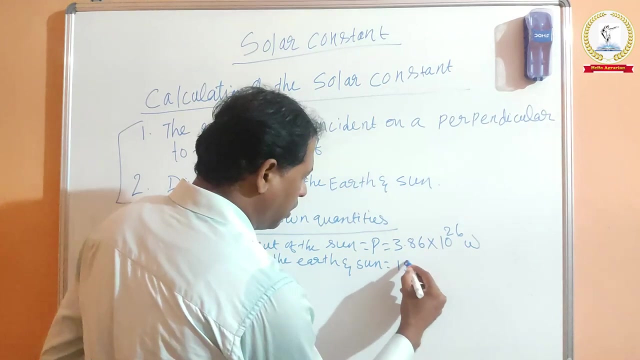 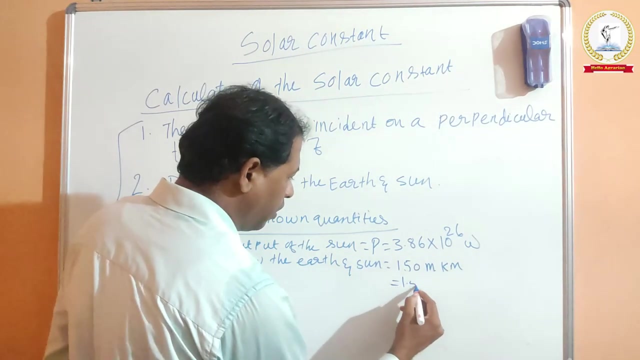 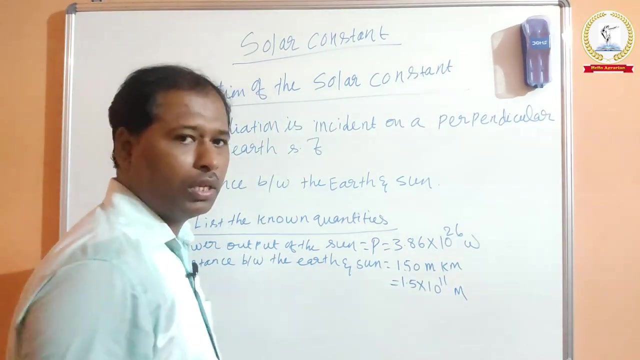 3.86 into 10 to the power of 26 watts. So this much amount of energy released by the sun. The second one is that distance between the earth and sun. Distance between the earth and sun That we already knows, About 150 million kilo meter, or you can say 1.5 into 10 to the power of 11 million. 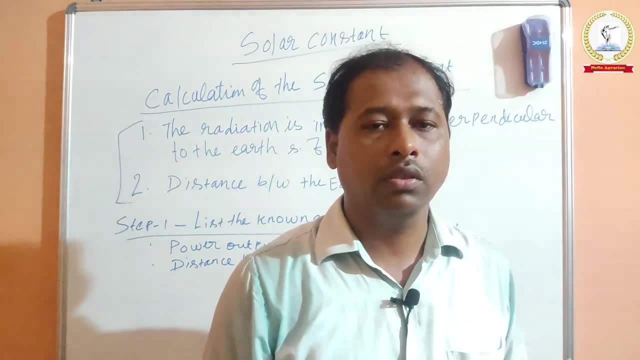 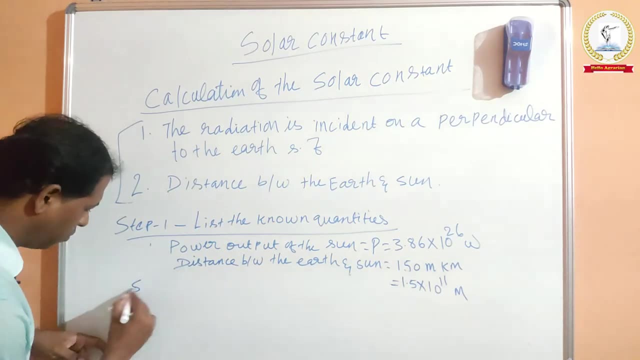 So by this way we can calculate the solar constant In step two model. the scenario using geometry Step two: 1., 2., 3., 4., 5., 6., 7., 8., 9., 10.. 11., 12., 12., 13., 14., 15., 14., 15., 16., 17., 18., 19., 20., 21., 22., 21., 22.. 23., 24., 25., 26., 27., 28., 29., 29., 30., 31., 31., 32., 32., 33., 34., 35., 35.. 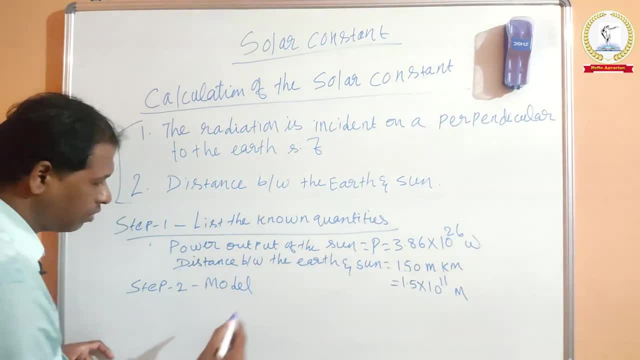 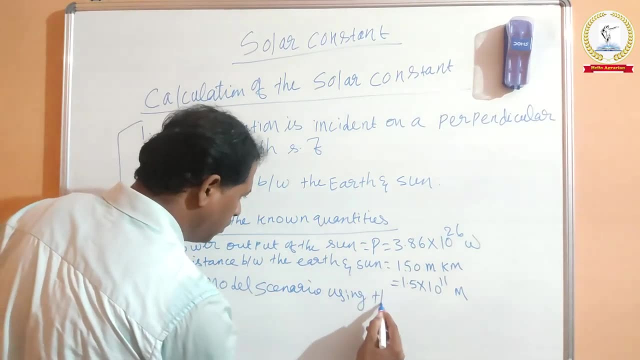 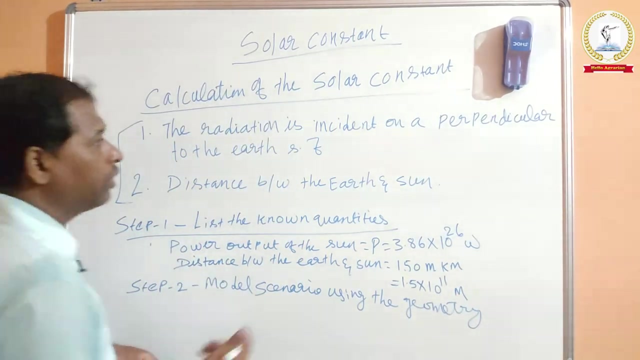 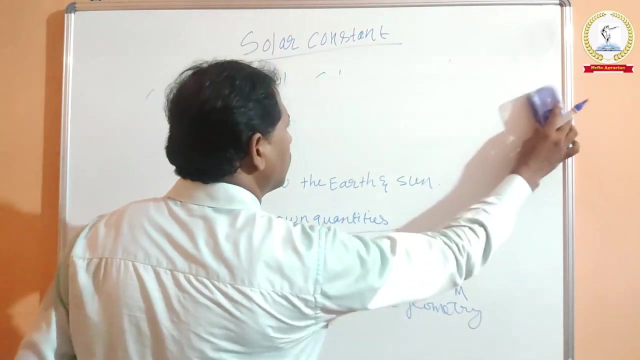 36., 36., 36. 37., 38., 38., 39., 39., 39., 39., 39., 40., 40., 40., 41. So for this I can delete this one. 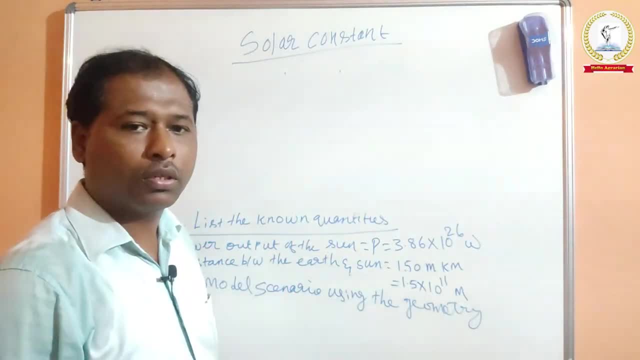 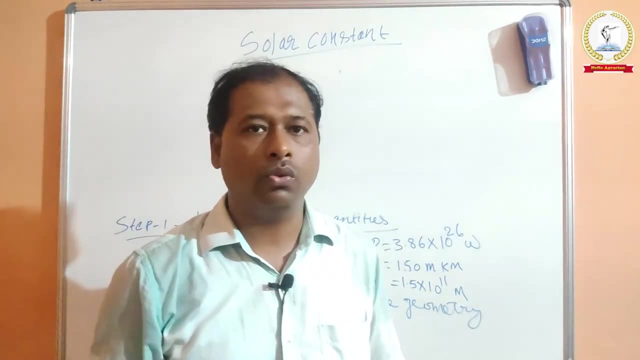 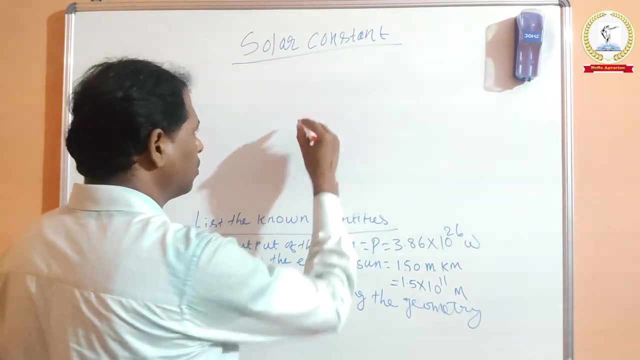 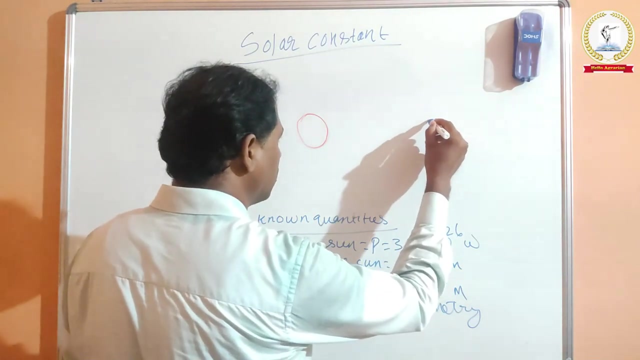 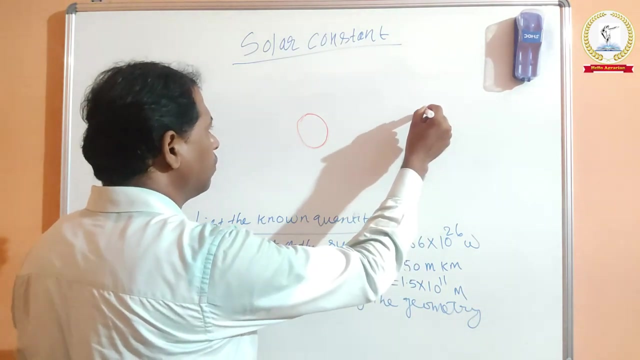 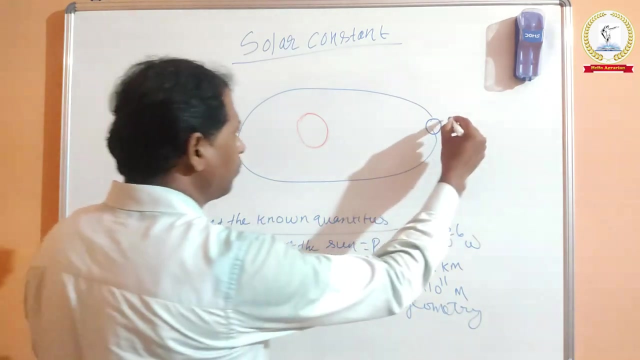 So as light release the surface of the sun, it begins to spread out uniformly through the spherical cell. So, for an example, this is the sun and this is the earth. So this the earth, The earth revolves around the sun in an elliptical orbit. 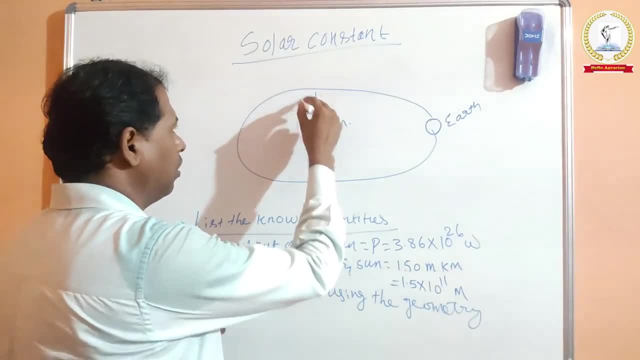 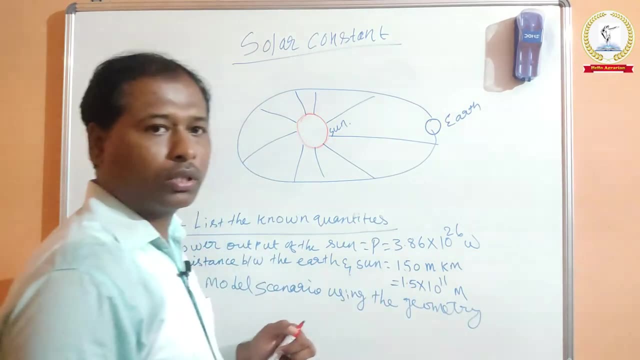 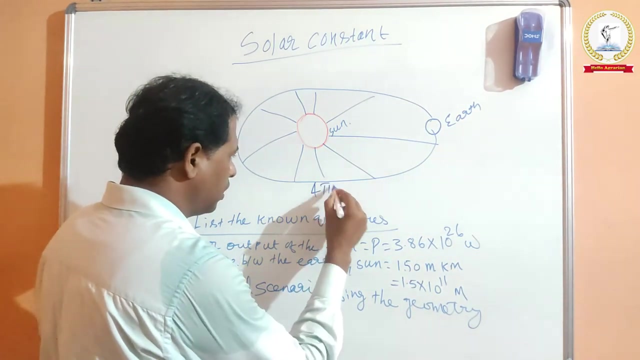 As light release from the surface of the sun, it spread out uniformly through the spherical cell. So the surface of the spherical cell is like this. 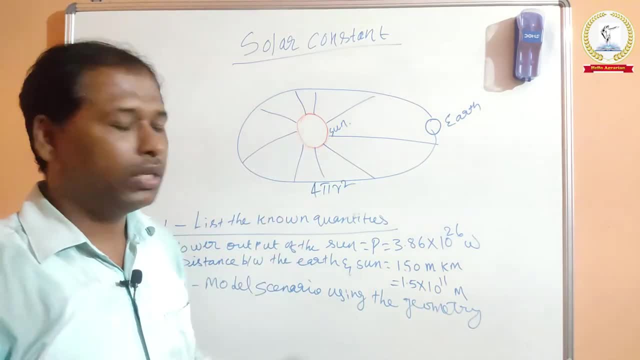 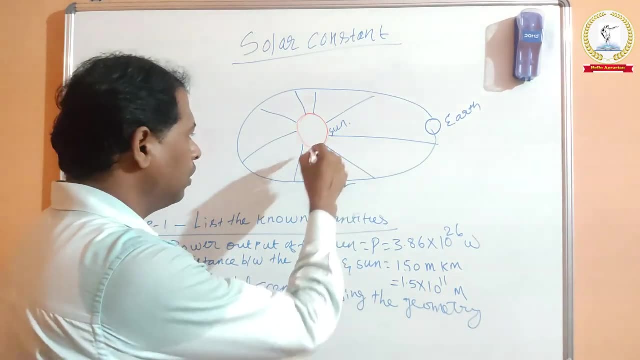 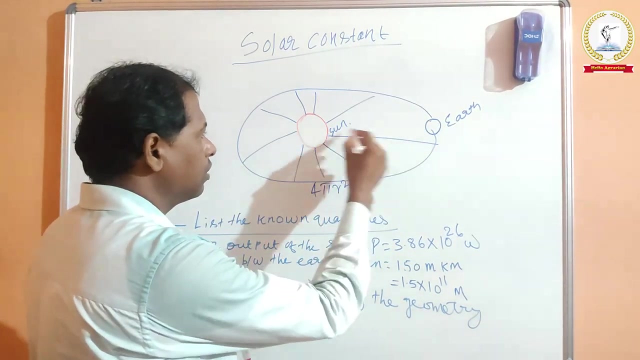 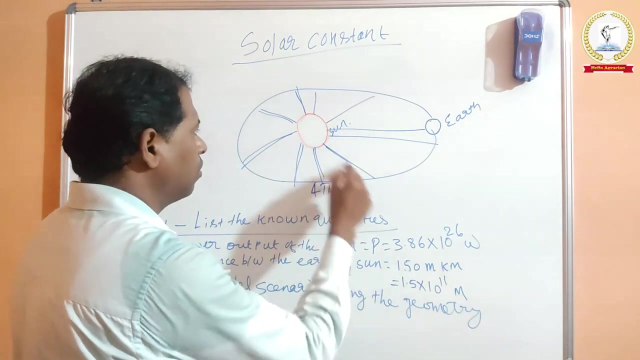 The surface area of the sphere. The surface area of a sphere is 4 by R squared, And the radius of the radius of this sphere is equal to distance between sun and earth. The radius of this sphere is equal to the distance between sun and earth. 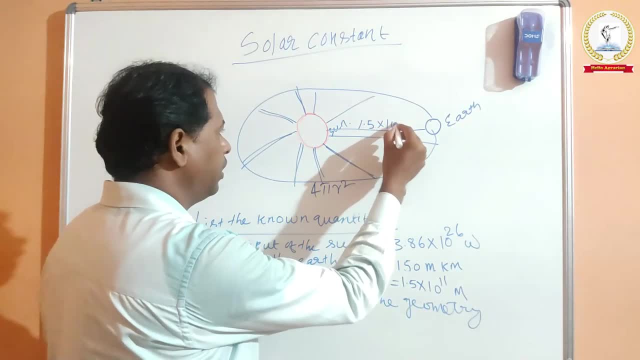 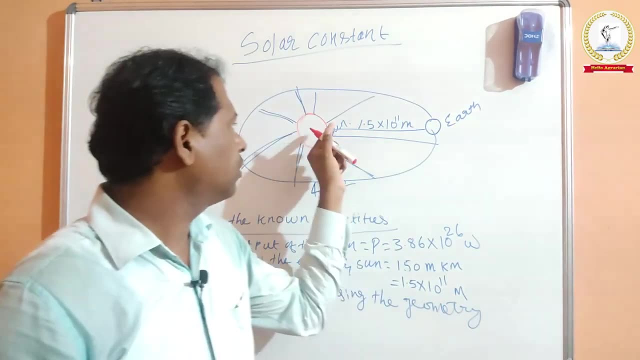 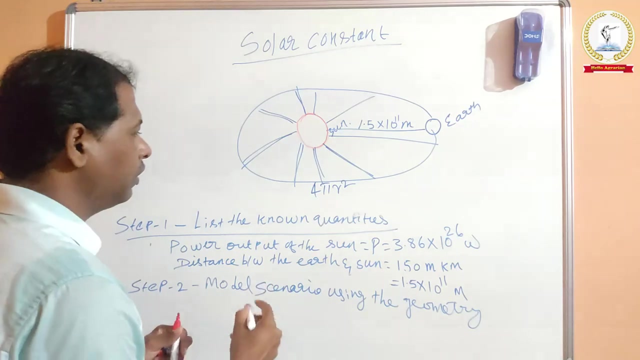 That is is 1.5 into 10 to the power of 11 million. So right now we discussed this 1.5 into 10 to the power of 11 million- And the power of the sun. the power of the sun is 3 point. 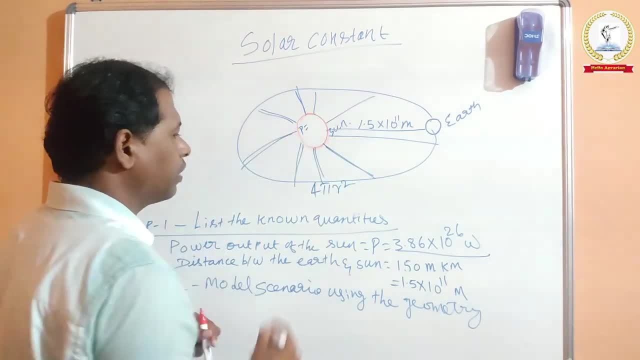 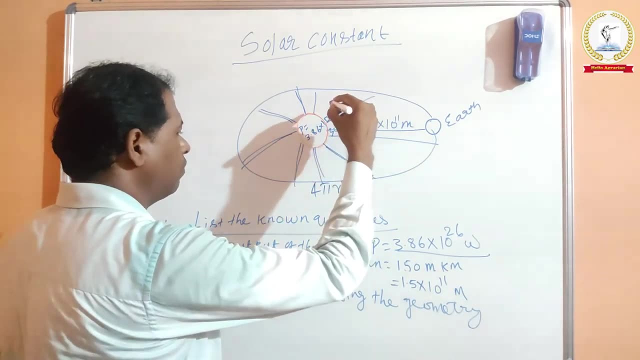 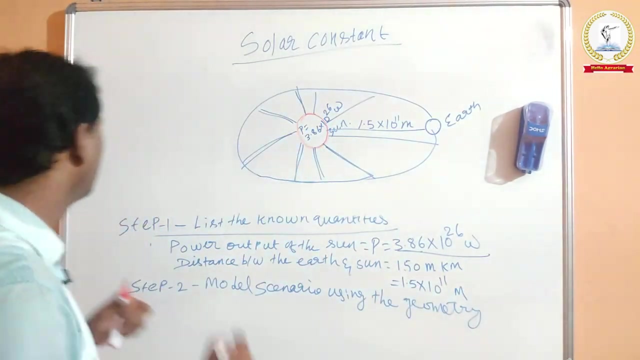 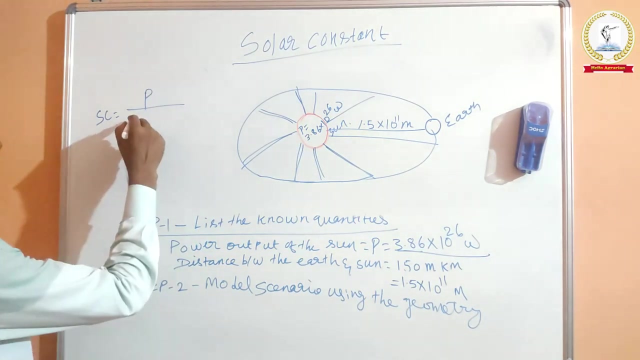 I can write over here. Okay, the power of the sun is 3.86 into 10 to the power of 26 watt. Okay, then now we can write the equation. solar constant equation is power output of the sun divided by 4, by r squared. Okay, so this value. 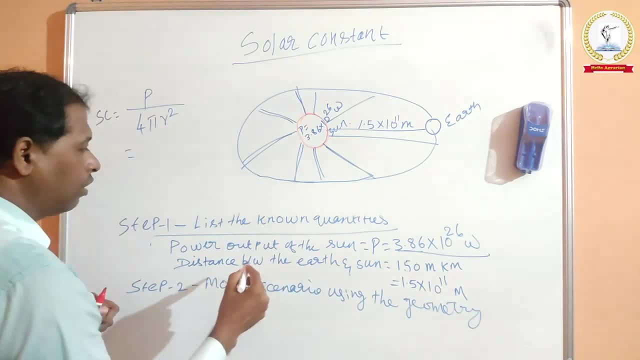 is 1.5 into 10 to the power of 11 million. So right now we discussed this, 1.5 into 10 can substitute. So this p, this power of the output of the sun value, is 3.86 into 10 to. 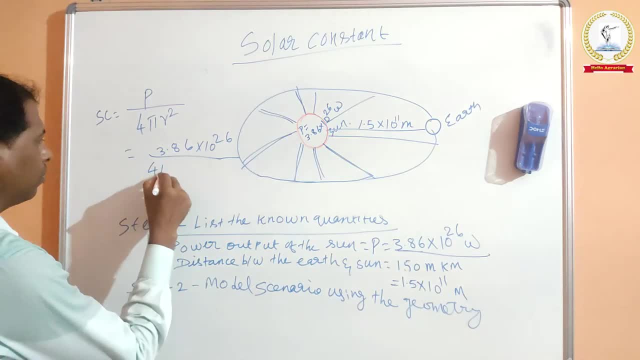 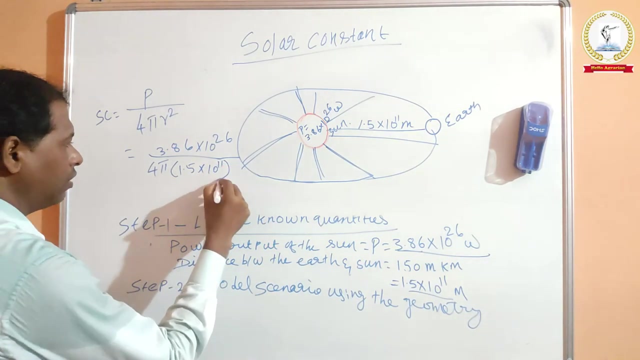 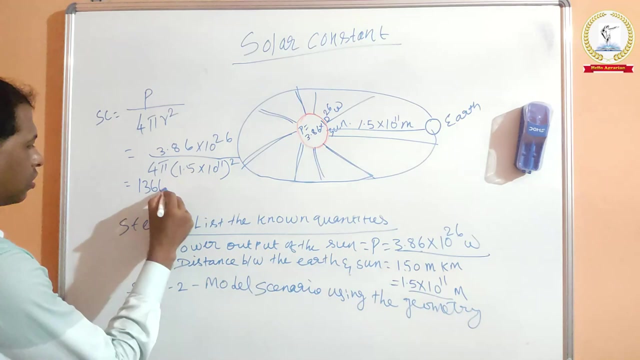 the power of 26 and 4 by the distance between earth and sun is 1.5, 1.5 into 10 to the power of 11 square. So you will get 1366 watts per square meter. even you can express in: 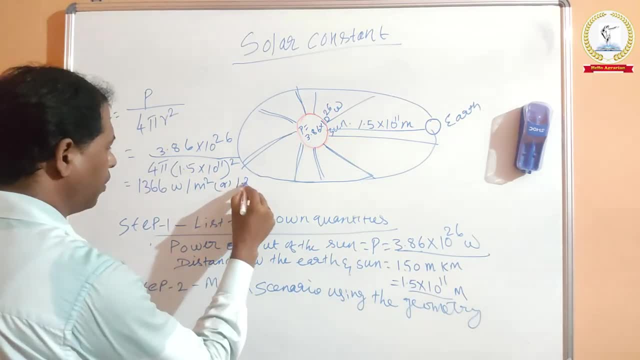 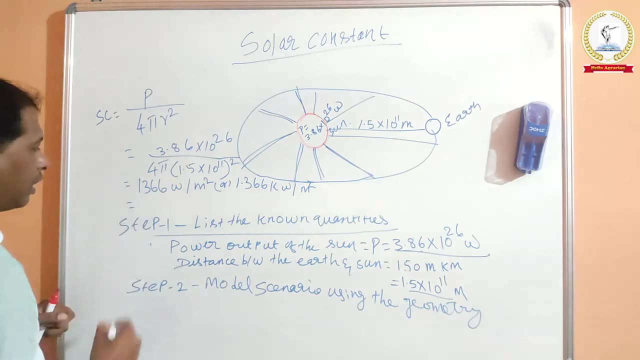 or 1.366 kilowatts per square meter. In terms of calorie, you can express in 1.94 kilowatts per square meter. So this is called solar constant value. So solar constant value ultimately is 1366 watts. 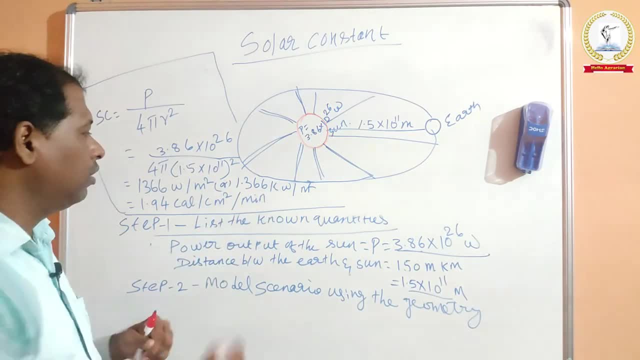 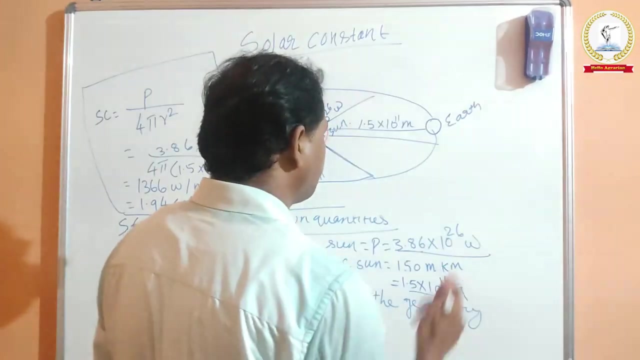 per square meter. In terms of kilowatt, it is 1.366 kilowatts per square meter. In terms of energy, it is 1.5, 1.34 calorie per square centimeter per minute. So for an example: 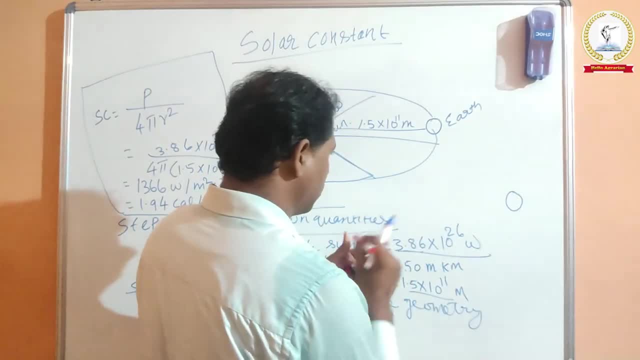 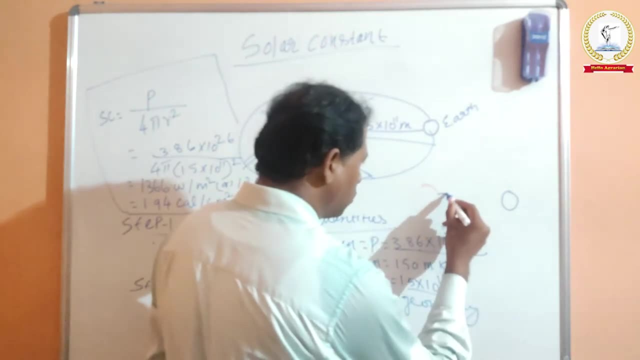 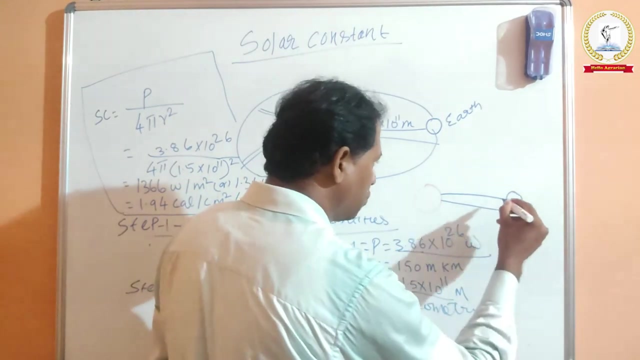 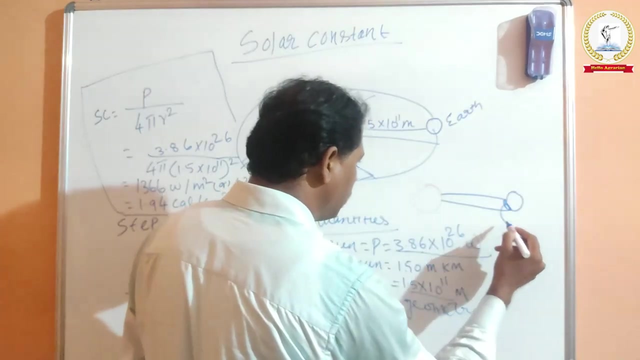 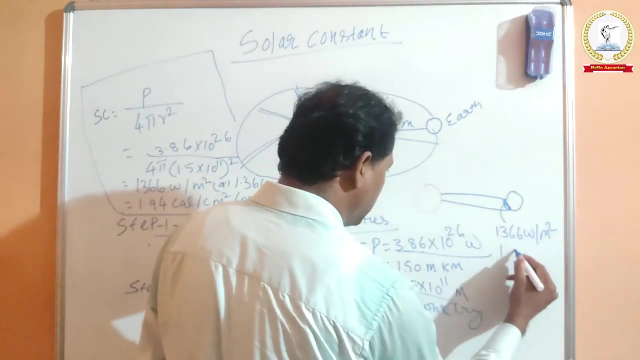 suppose this is the earth and this is the sun. The amount of solar radiation falling on the earth surface, that means top of the atmosphere in a particular unit area, in a particular unit area. So that is equivalent to 1366 watts per square meter, or you can. 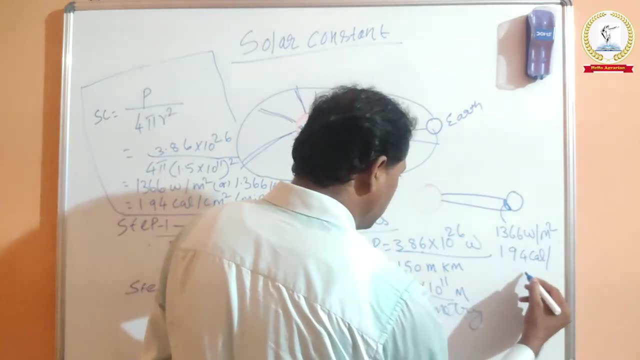 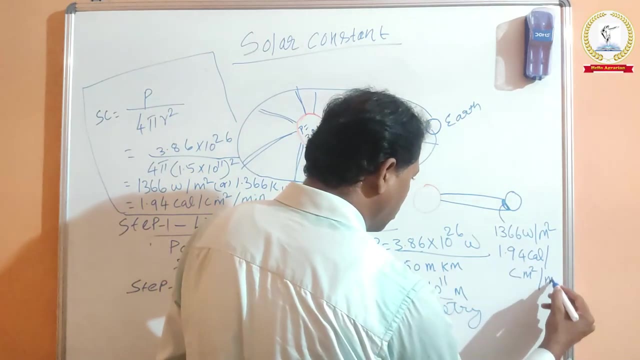 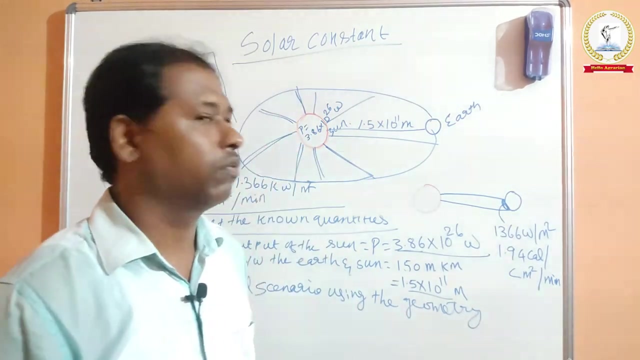 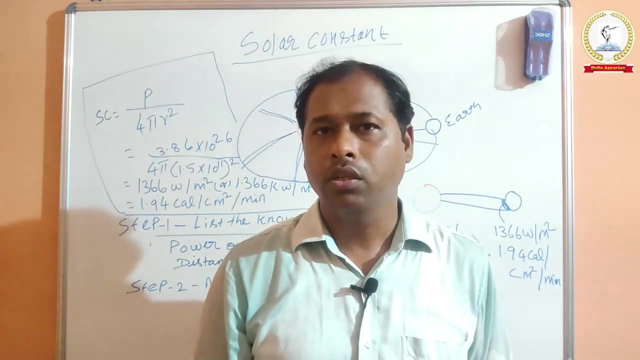 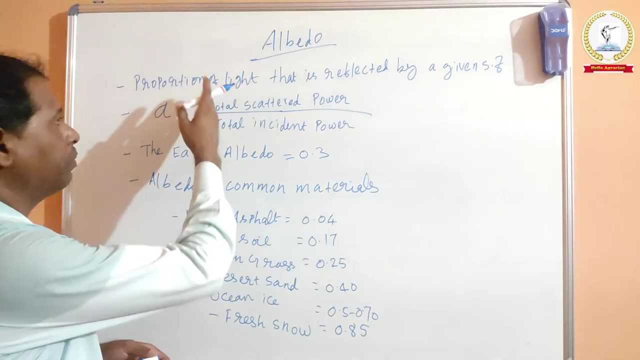 say 1.94 calorie per square meter per- sorry, per square centimeter per minute. So it is called solar constant value. I hope you all understand about this solar constant, how to calculate this solar constant. Next one is albedo. Albedo means the proportion of. 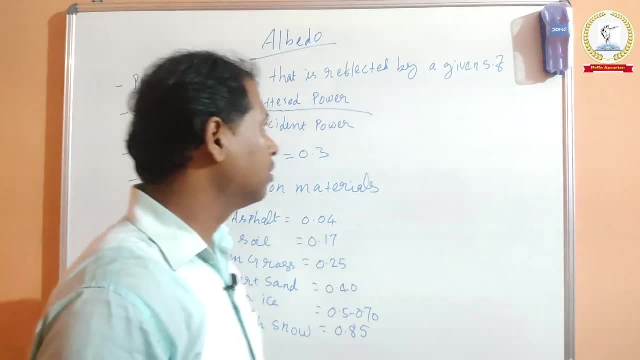 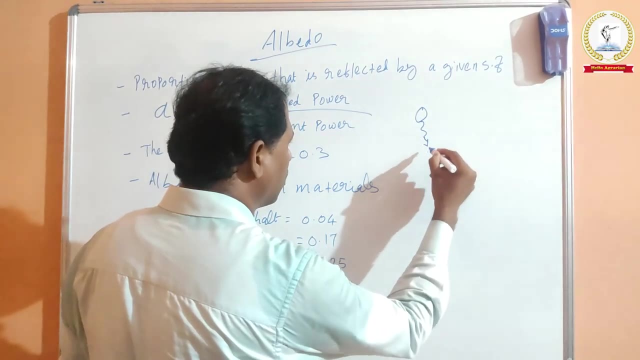 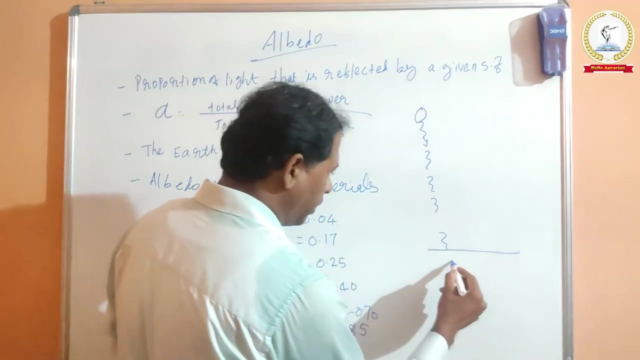 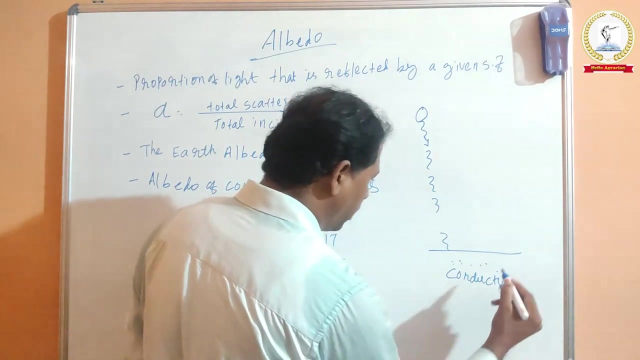 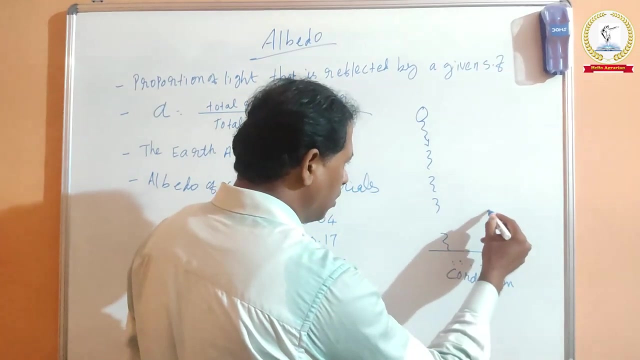 light that is reflected by a given surface. as we know that Sun emits a shortwave radiation, are positive or negative. Once reach on the surface, the soil gets heated up first. that is conduction process take place. Once soil got heats up, then it emits in a long wave radiation. 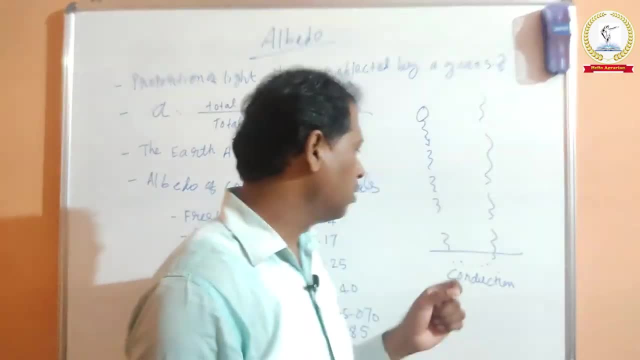 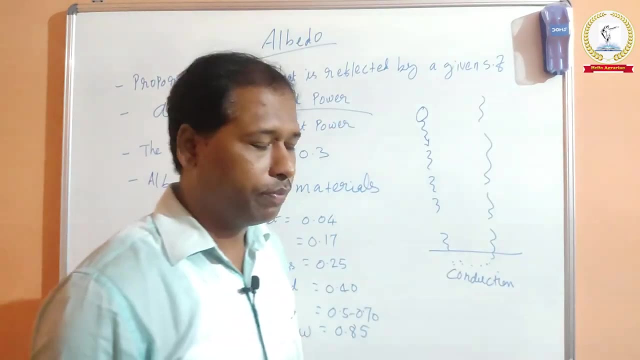 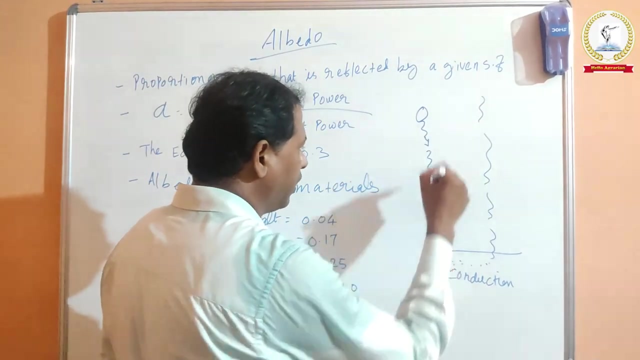 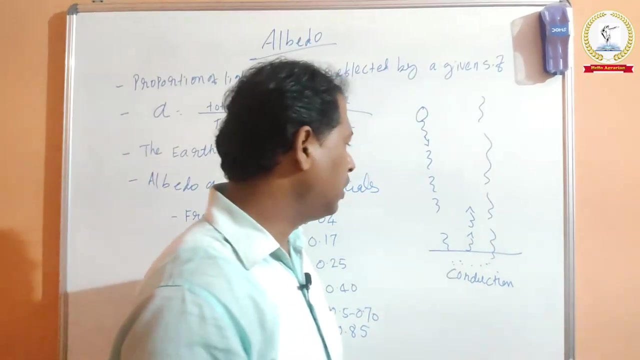 So this is commonly held in our soil. First, the sun emits short wave radiation and ground emits long wave radiation because our ground is a radiation body. In some case this short wave radiation reflected as a short wave radiation itself, without changing any its quality. that is called albedo. 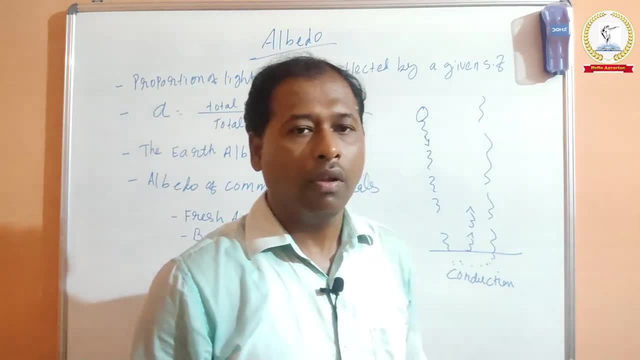 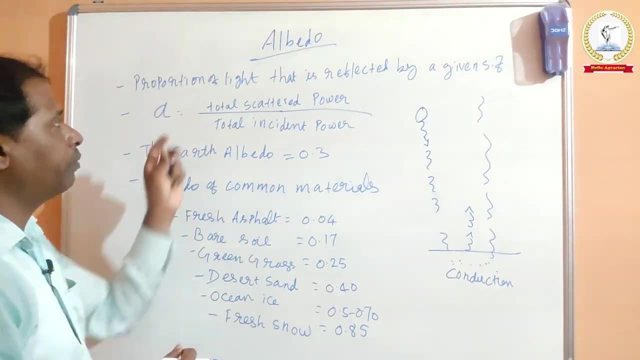 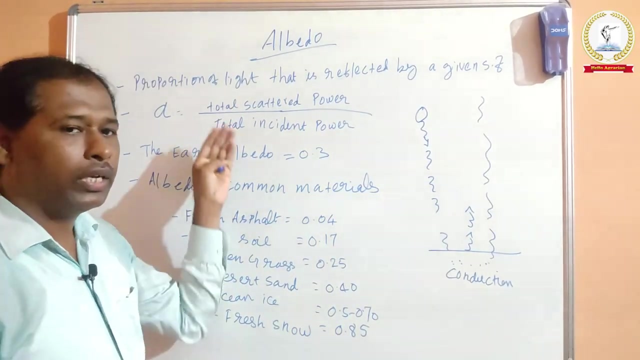 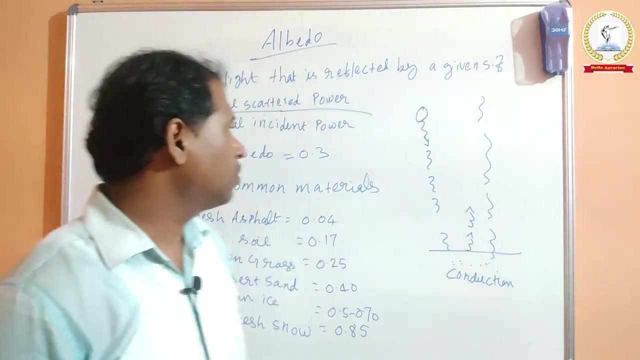 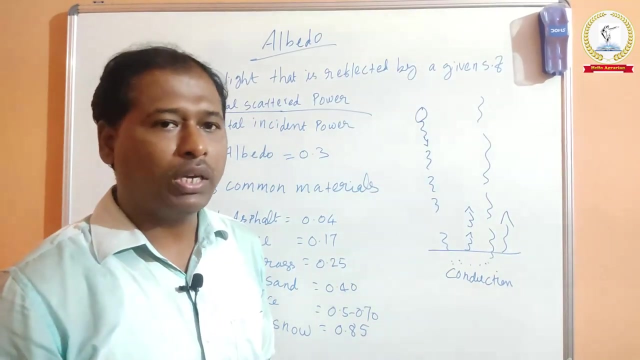 The reflection of the same radiation without changing any its quality. So that is called albedo. So that is proportion of light that is reflected by a given surface. So it can be calculated as total scattered power upon total incident power. So out of incident power, how much power scattered without changing in its quality? 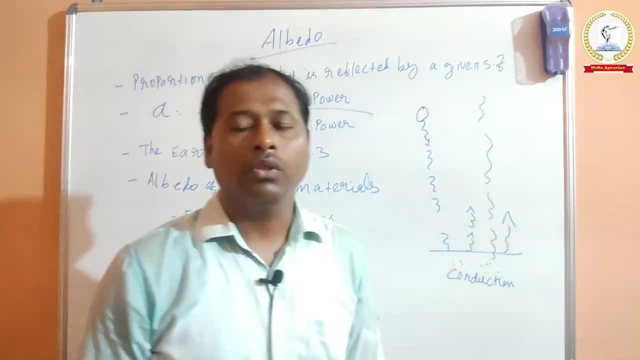 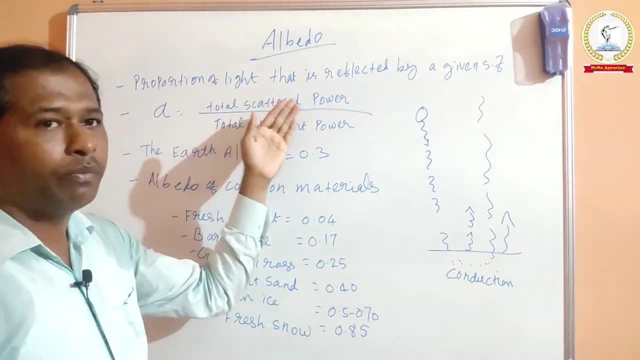 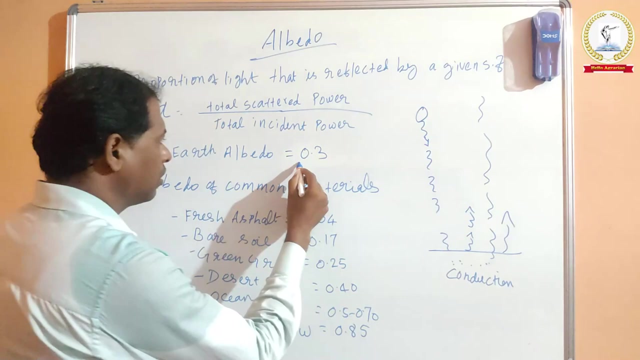 So that is called albedo. So that is called albedo, So that is called albedo. So you can define more specifically that the ratio between the scattered total scattered power to the total incident power, The earth albedo, is 0.3.. 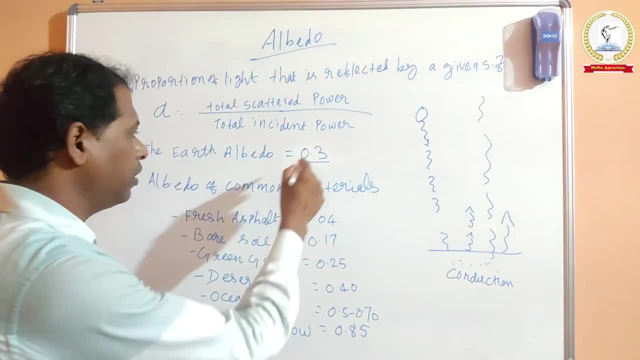 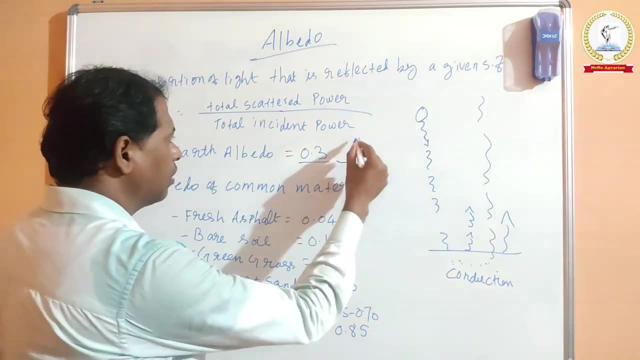 Earth albedo is generally taken to be 0.3, which means 30% of the sun rays that is reflected back to the atmosphere without changing in its quality. So you can define more specifically that the ratio between the scattered total scattered power to the total incident power. 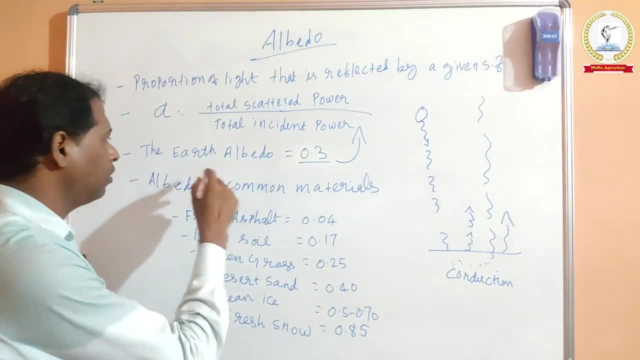 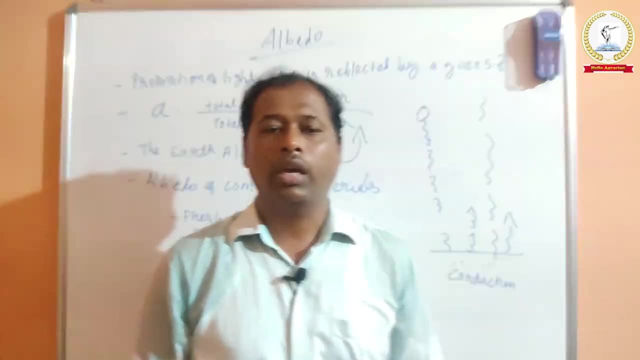 The ratio between the scattered total scattered power to the total incident power without changing in its quality. So the general albedo for the earth is 0.3.. You see, the earth albedo varies daily and depend on various factors like the latitude. 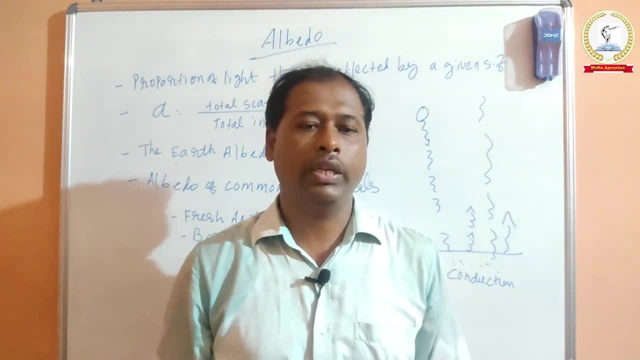 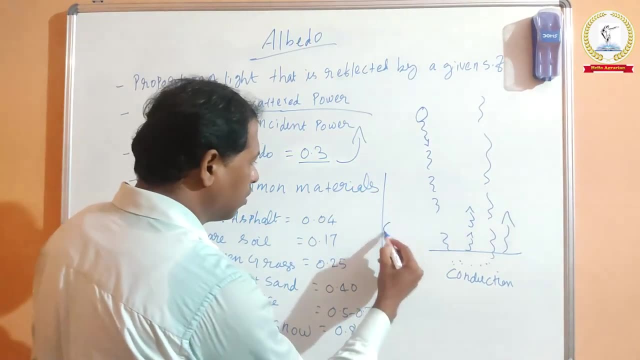 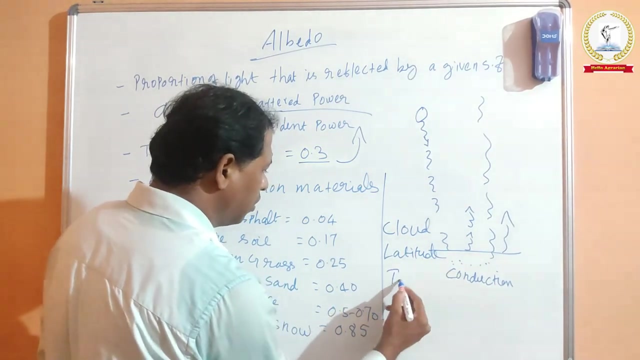 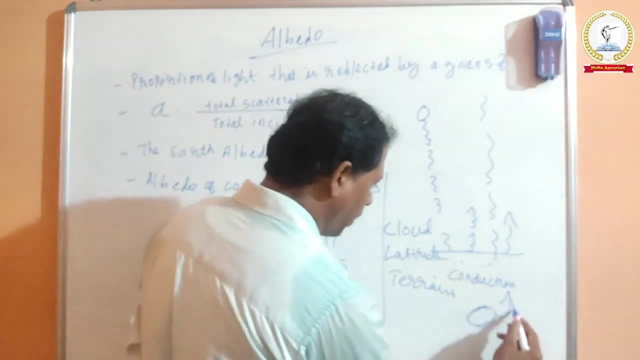 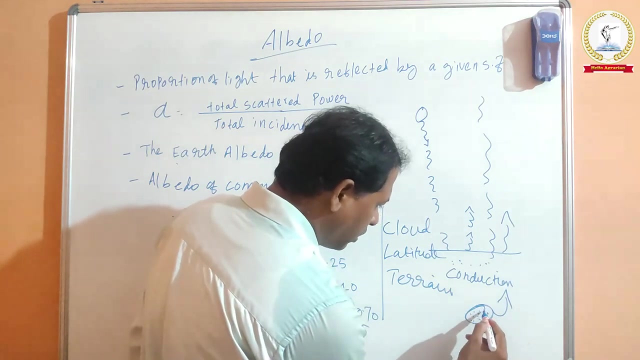 cloudiness and even Terrestrial influence also. So it may vary on the front and rear of the earth. So it may vary upon cloud and terrain influence. okay, if there is thick clouds, then more reflection take place, because this clouds contains more ice crystals and this ice crystals reflect the radiation. okay, 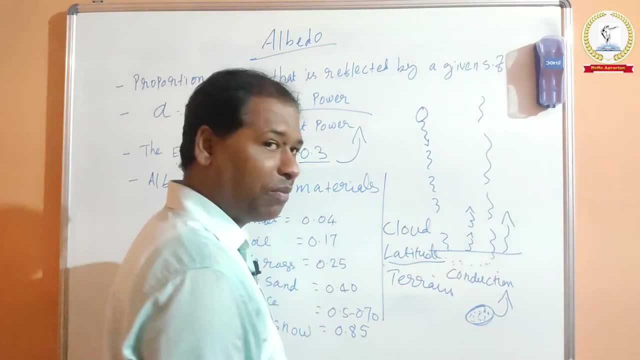 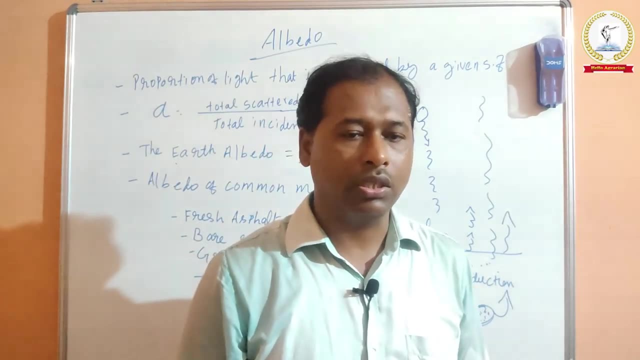 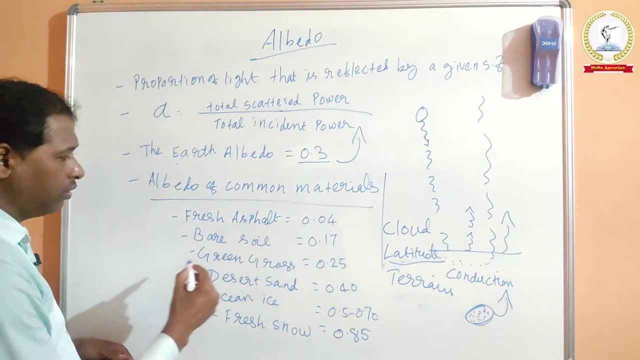 so latitude also vary. the albedo right, mid-latitude, produce more albedo as compared to equator region. so I have given Albedo of common materials. you see, bread spot has 0.04, bare soil is 0.17 and green grass 0.25. for desert: 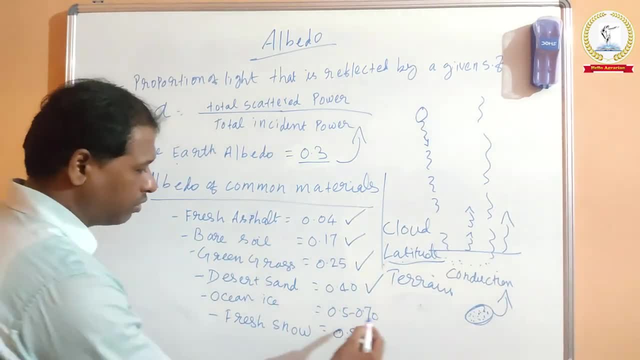 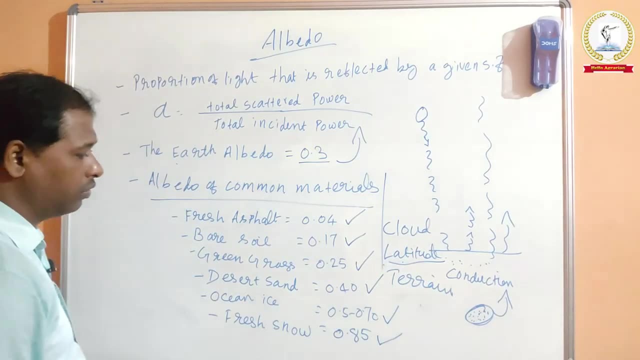 city used as an albedo for albedo better as compare to equator region. so I have given common materials. you see fresh asphalt as 0.04, bare soil is 0.17 and green grass 0.25, sand it is 0.4, ocean ice 0.5 to 0.7 and for fresh snow it is 0.85.. 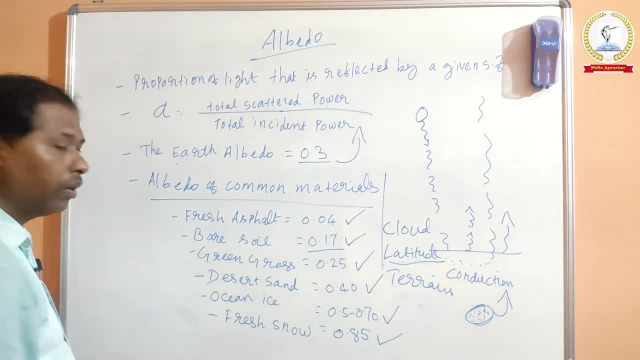 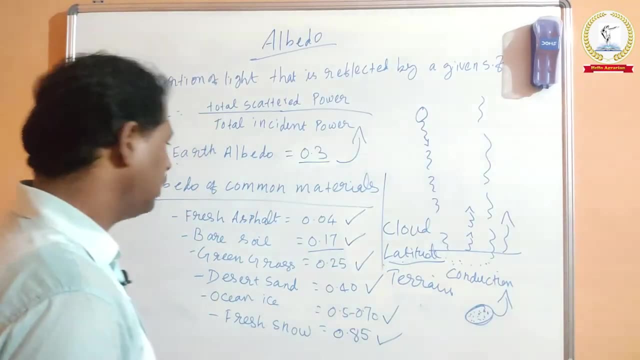 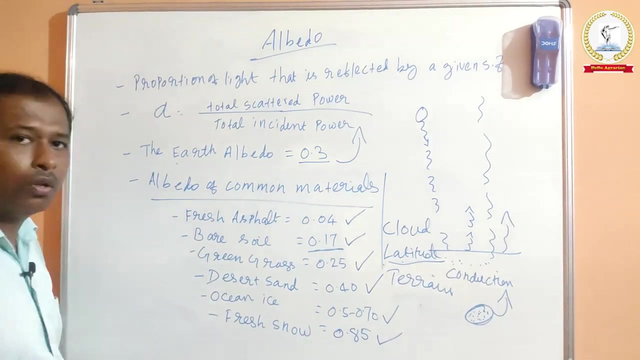 So among these we found the low value for bare soil, because the soil able to observe more amount of radiation. that's why their reflection is low. So it is average value of bare soil is 0.17, whereas fresh snow has 0.85, it is more among. 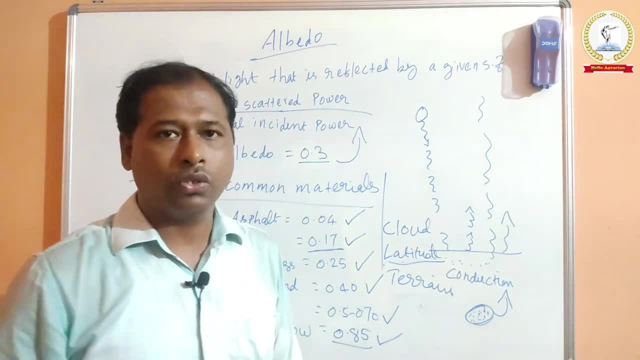 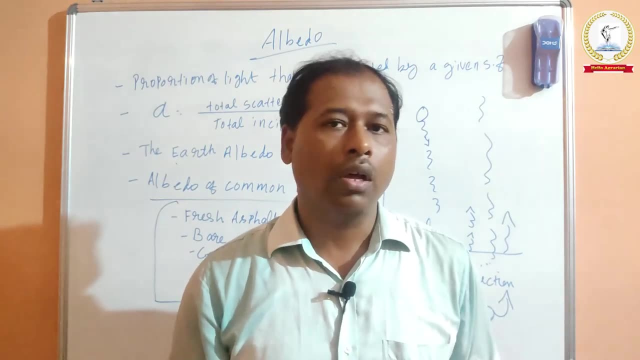 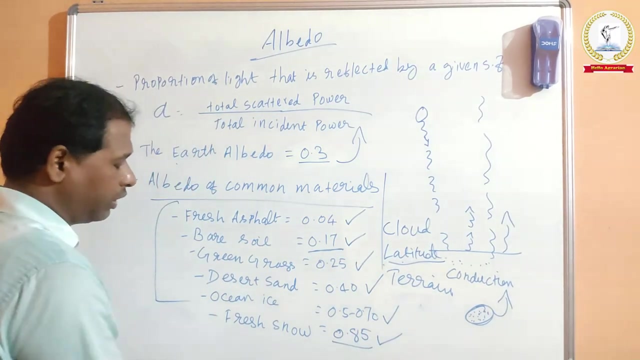 them because the fresh snow actually white color and it reflects more as compared to absorption. So that's why their reflection, due to the more reflection, The Albedo rate is more. for fresh snow, whereas you see green grass, again it is low value. that means it observe more amount of radiation. similarly, the fresh aspart sheet- fresh aspart. 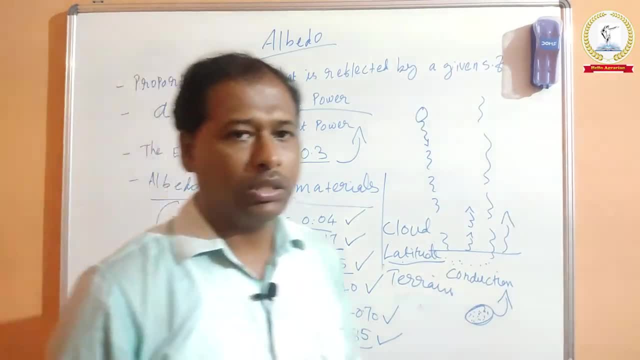 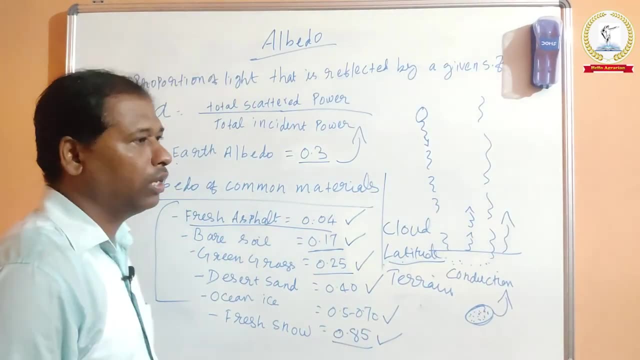 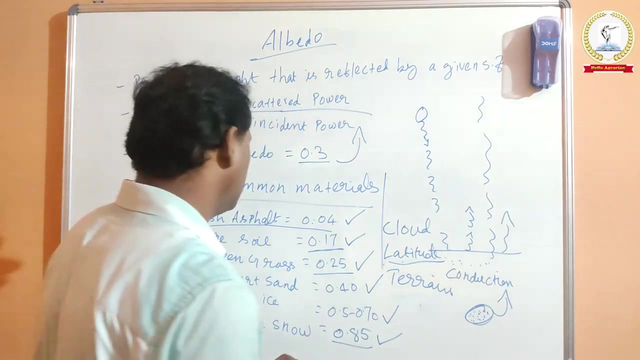 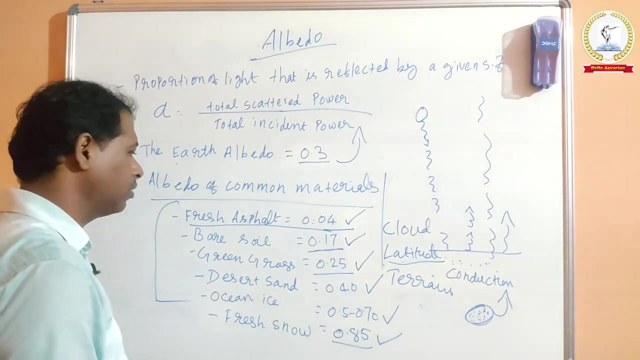 sheet it is 0.04. that means entire amount of solar radiation observed by this aspart sheet and that's why a house Made up of aspart sheets so they feel more warm because it observe more amount of solar radiation and cause warm of that inside. 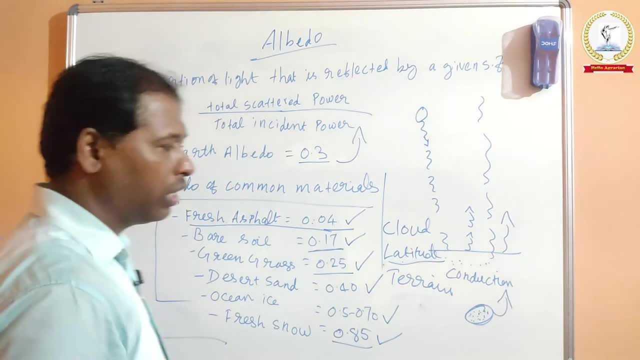 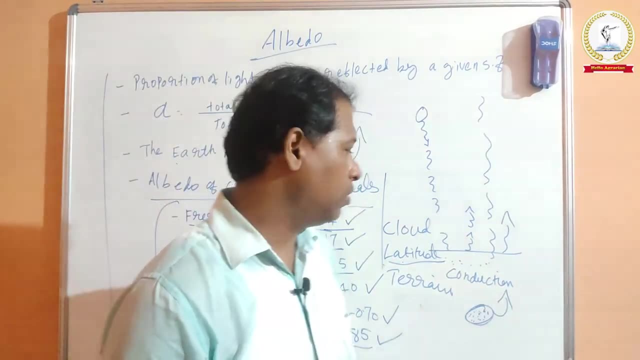 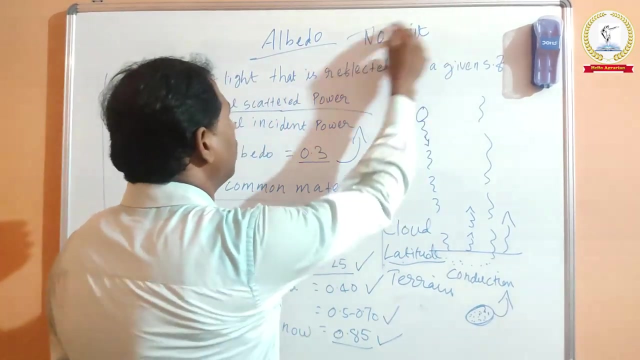 So this is all about albedo. this is all about albedo. you see, here albedo has no unit because it is the ratio of power. So there is no unit for albedo. So, So, So, So there is no unit for albedo because it is ratio of power. 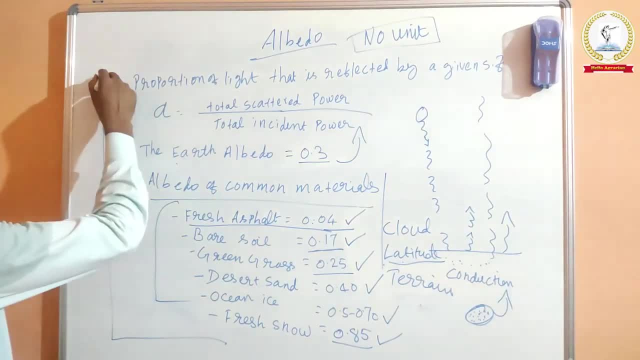 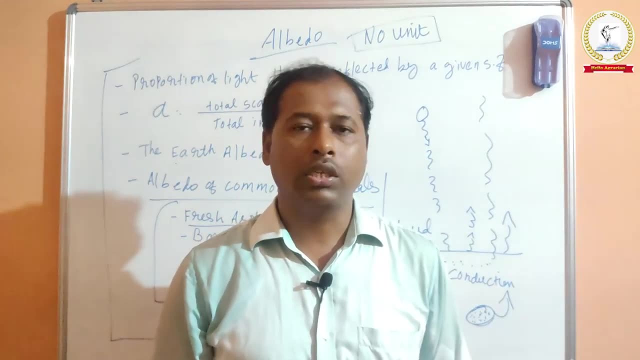 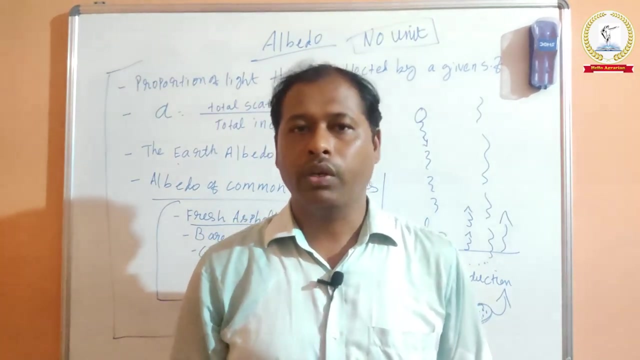 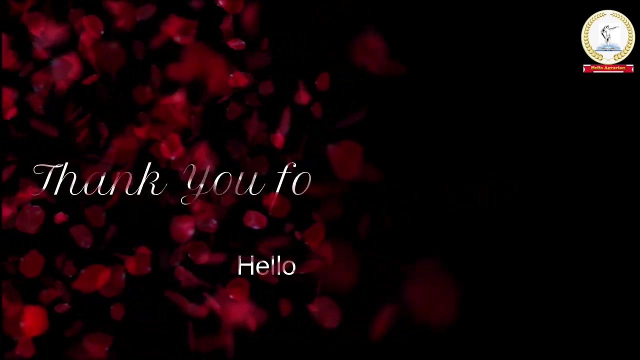 So this is all about albedo. I hope you all understand about this solar constant and albedo, what we discussed in this video. If you have any query, you can give the. you can give your valuable comments in the chat box. Thank you you.